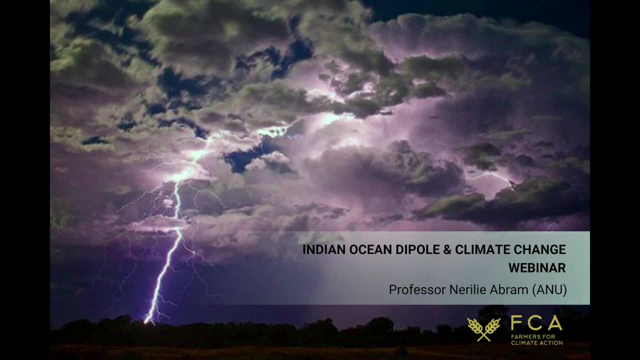 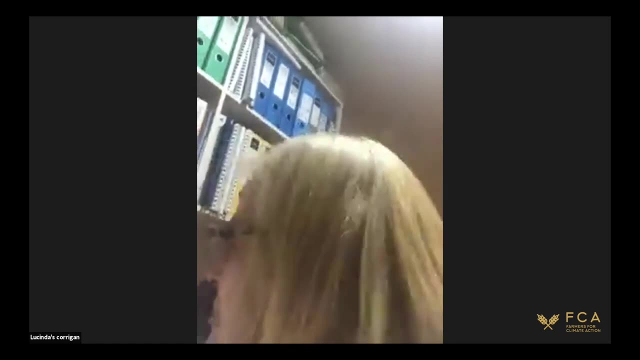 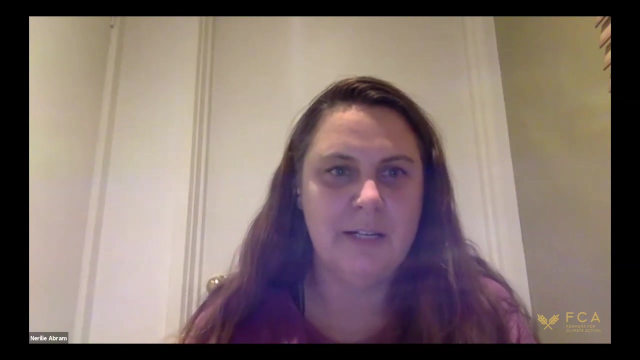 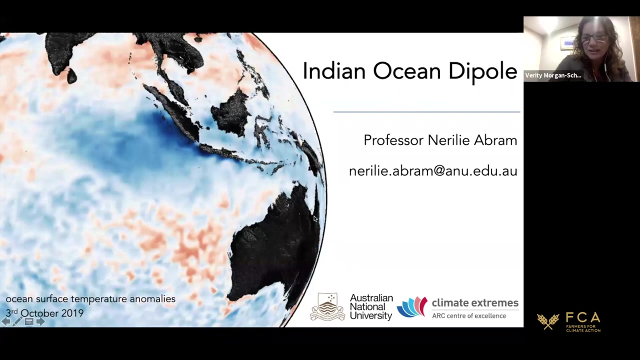 If you're interested in your talk tonight about the Indian dipole and over to you. Okay, thank you very much. I'm just going to start sharing my screen, Neralee. just before you start, I'll just let everyone know that it's now being recorded, so. 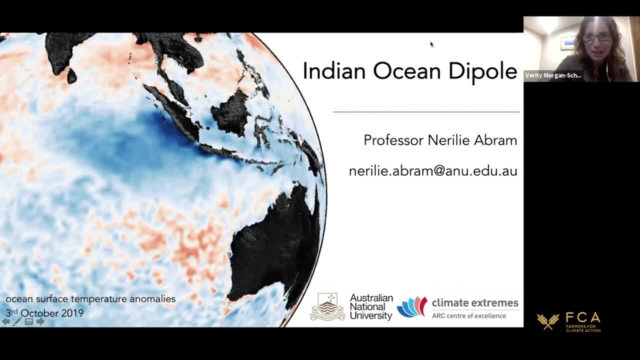 that we can share this with everyone who isn't able to dial in tonight. Neralee's presentation will be available afterwards. We were hoping to send it out with the email and unfortunately it was too big for our system to send. So we'll work that out tomorrow morning and get it through. 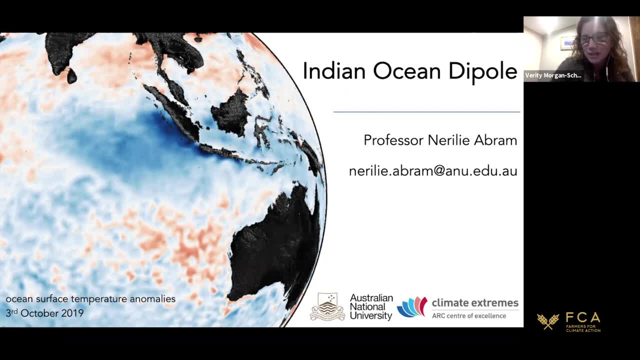 to all of you, And any questions, please just pop them in the chat box so that we don't have people trying to speak over the top of each other, and then we'll get on with it. Thank you so much, Neralee Great, thank you very much. Thank you for the invitation to speak. 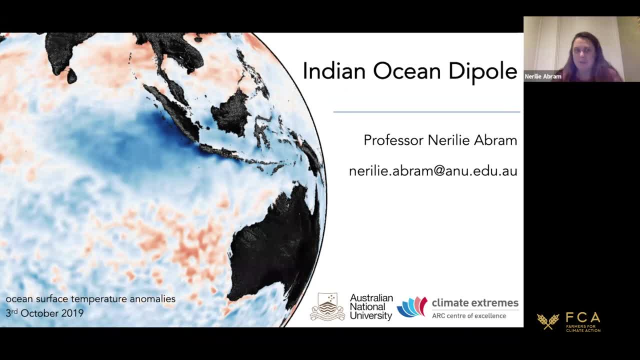 The farming community is a community that I haven't had a chance to speak to sort of as a group before. I have had some experience in working with governments to convey scientific information to them, But the work that we do is aimed at trying to understand. 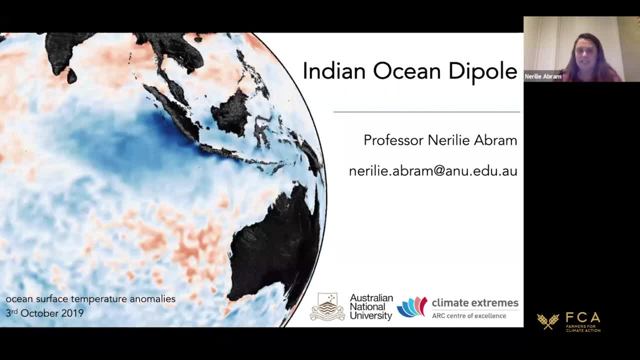 what causes variability, particularly in Australia's rainfall, And so we're very conscious that the information that we're providing, the research that we're doing, is quite relevant for your communities, or we hope that what we're doing is relevant and useful for 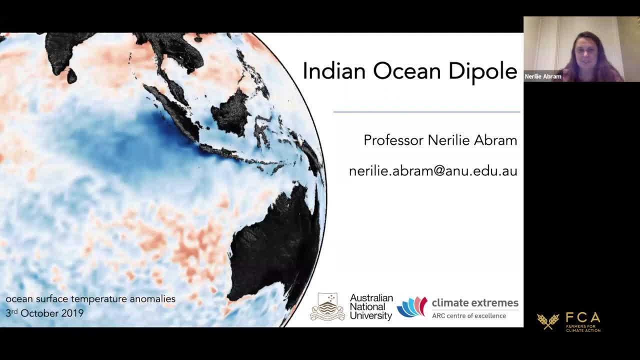 your communities, So it's really nice to be able to speak to you today. So what I'm going to be talking about is the Indian Ocean Dipole and, specifically, the work that I've been doing with quite a large team of people to look at ways that we can reconstruct the variability. 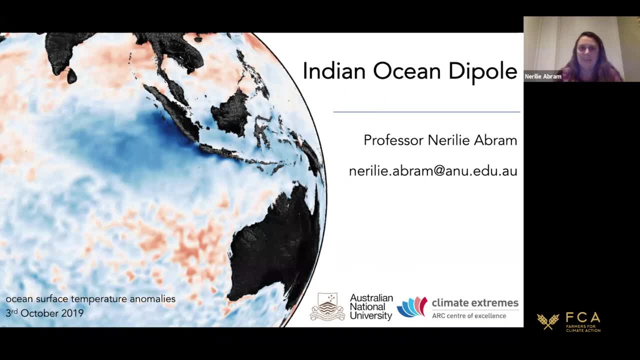 of this climate phenomenon back in time, back over the last millennium, and to then use that to give context to our observational records and our climate model projections of the Indian Ocean Dipole, so that we can have more confidence in being able to see how this system behaves. and 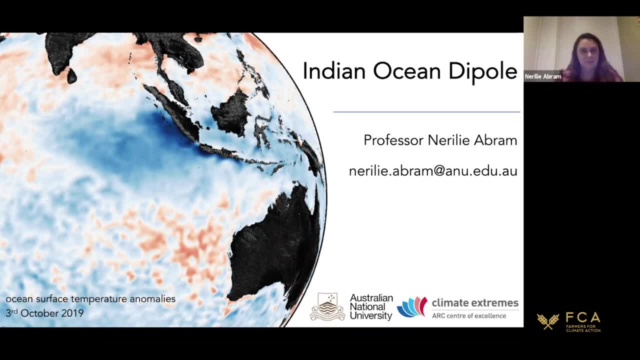 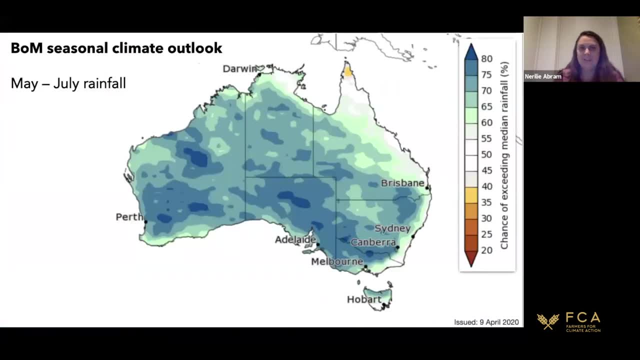 how it's being altered now because of human-caused climate change, Right? so I thought that I'd start on this very positive note, actually, which is the Bureau of Meteorology. it's the most recent seasonal climate outlook, so the rainfall outlook for May to July, and we can see lots of areas of 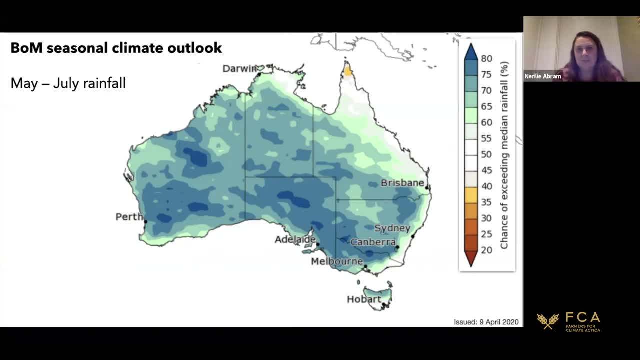 blue, so indicating that most of Australia has a good chance of exceeding the median rainfall that you'd expect for this time of year. And the reason that I wanted to start here is that what you can see in this image is that rainfall patterns are really extending from the northwest of Australia and then 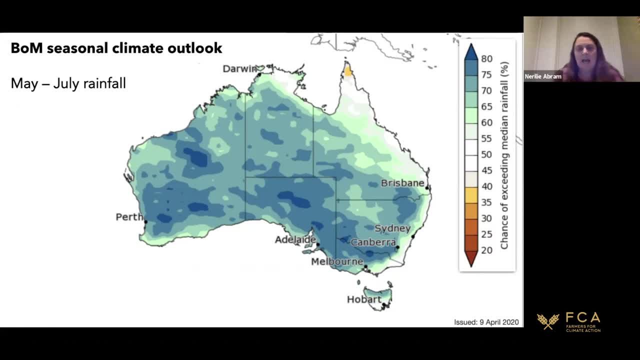 sweeping across Australia down towards the southeast, And just this visual here. I think already just by looking at that intuitively you can see that this area to the northwest of Australia is a really important area when we think about where our rainfall comes from. 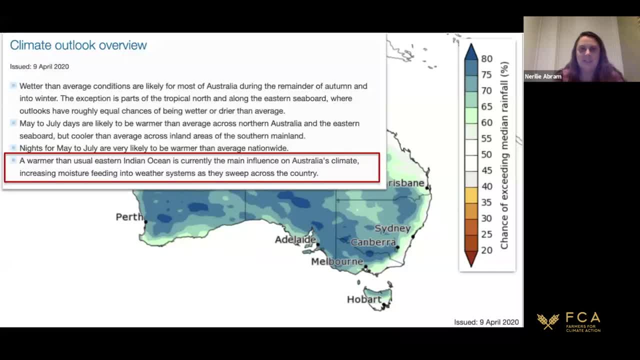 So that's the starting point and just the text that goes along with this, saying that a warmer than usual eastern Indian Ocean is that main influence that we're seeing on Australia's climate at the moment, And because that ocean is warm, it's feeding moist air into weather systems. 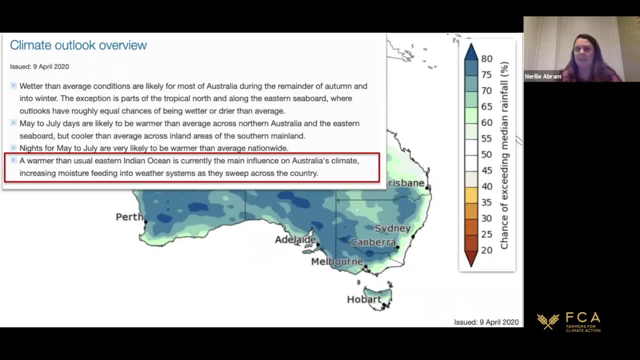 as they sweep across the country. So as we get these cold fronts traveling across the country, they're drawing down air from the northwest of Australia, and that air at the moment has a lot of moisture in it, and so that gives us an increased chance of getting rainfall. 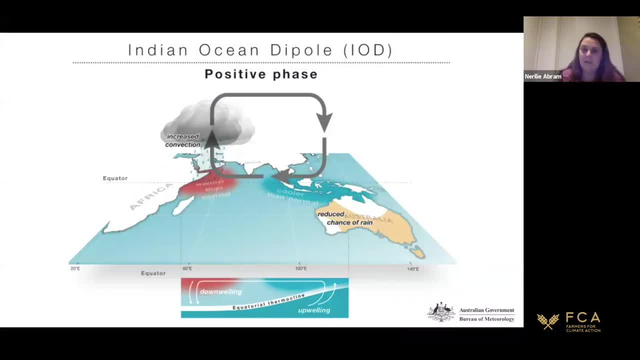 So I think the Indian Ocean Dipole- some of you may have heard of this before, others may not. It's a similar kind of climate process to the El Nino Southern Oscillation, which I think probably most people have heard of, but the El Nino operates in the Pacific Ocean and the Indian Ocean Dipole 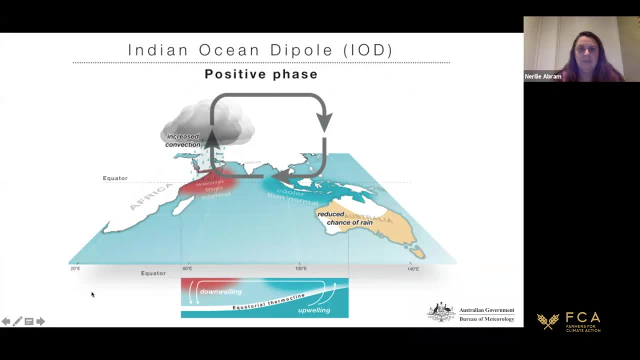 is operating in the tropical Indian Ocean. So it's an actual climate process- positive and negative phases- and what I'm going to be talking about mostly tonight is the positive phase of the Indian Ocean dipole. So when we have a positive phase, that's when we 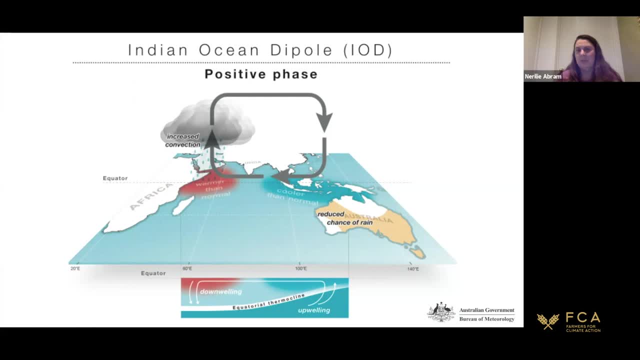 have water that is cooler than usual to the northwest of Australia, and when we have that cool water to the northwest of Australia, we've got less evaporation happening over the ocean, and so the air that would be drawn down across Australia doesn't hold moisture, or doesn't. 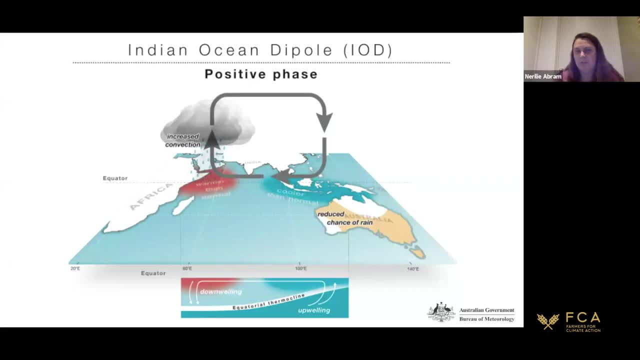 hold very much moisture, and so we have a reduced chance of rainfall in Australia when we have this positive Indian Ocean dipole. That's what we saw in 2019, and that was one of the contributors as to why Australia had its driest year on record in 2019.. These are just the maps from the Bureau. 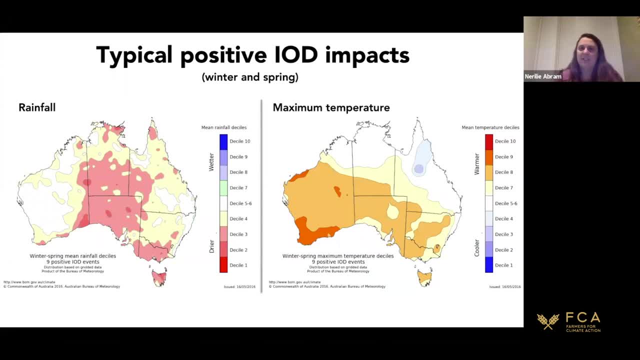 of Meteorology, just showing the typical impacts that you would expect when you have one of these positive Indian Ocean dipole events. So we see the impacts of the positive Indian Ocean dipole events in the winter and the spring and when we have a positive Indian Ocean dipole event, we have 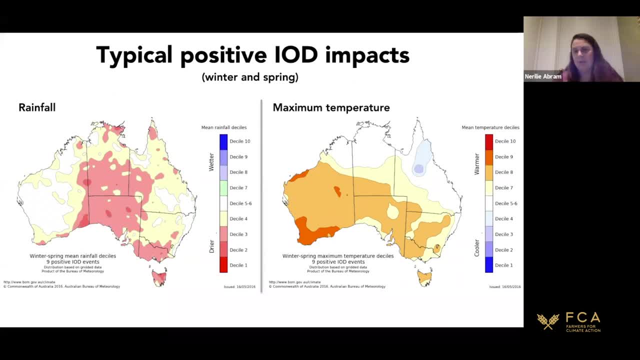 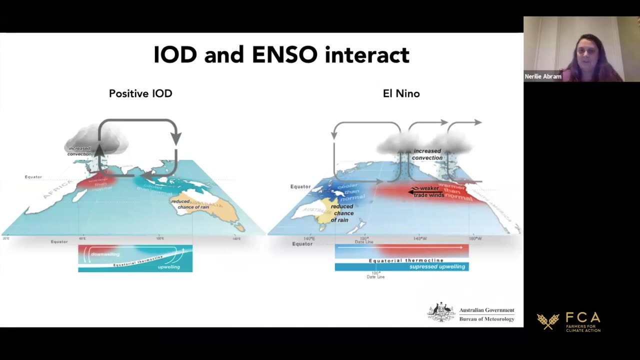 drier than usual conditions and we have hotter than usual conditions, particularly across the southern parts of Australia and particularly focused in the southeast. One thing that I just wanted to point out is that these climate processes don't operate in isolation. So we've got the Indian Ocean dipole. that's happening. 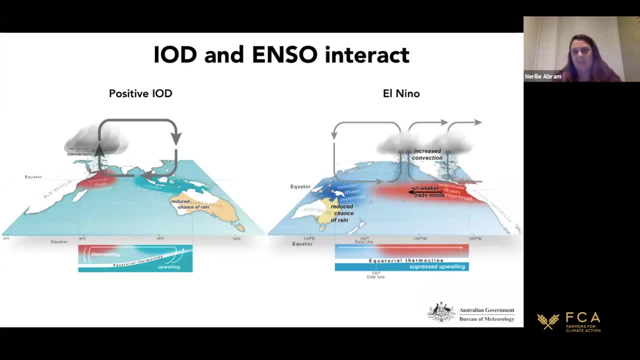 in the tropical Indian Ocean. we've got the El Niño phenomenon that's happening in the tropical Pacific Ocean and those systems interact with each other, particularly in the Indonesian area, and so when you have conditions, have El Niño conditions in the Pacific, you set up a situation where you're 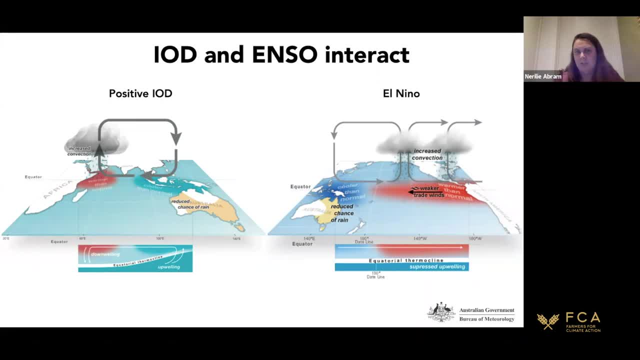 also more likely to have a positive Indian Ocean dipole event. So you can have these systems occur independently, but there is a high chance that you actually have them happening at the same time, And so when you have that situation you actually sort of have this double whammy for Australia's. 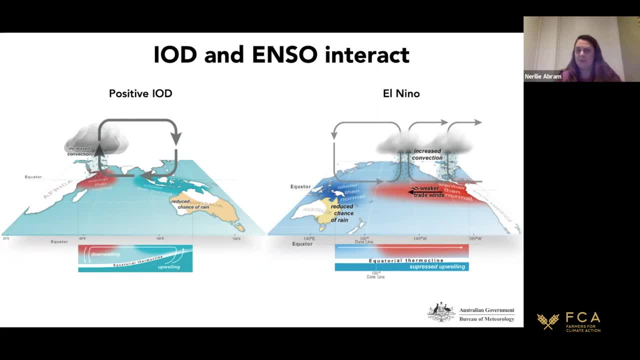 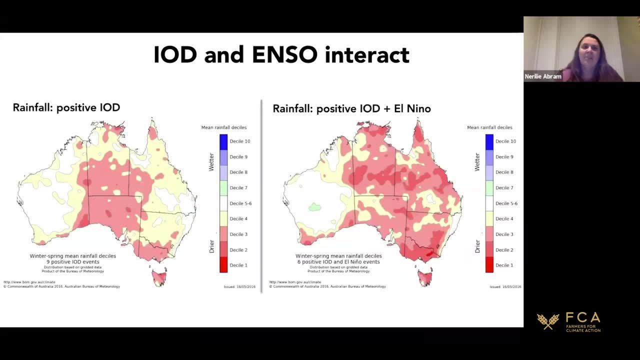 rainfall, in that you cut off one of your main moisture sources from the tropical Indian Ocean, but you're also cutting off that eastern source from the Pacific Ocean as well. And so when you have a positive Indian Ocean dipole event and an El Niño event at the same time, you have an even. 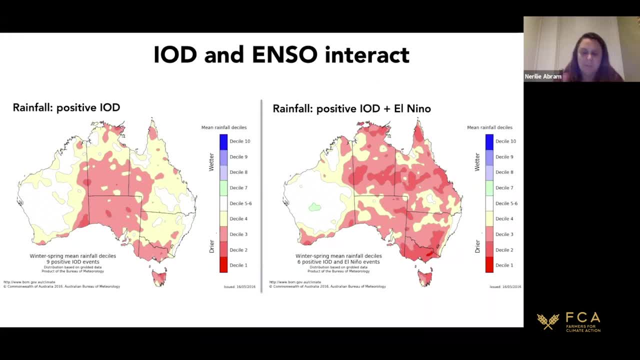 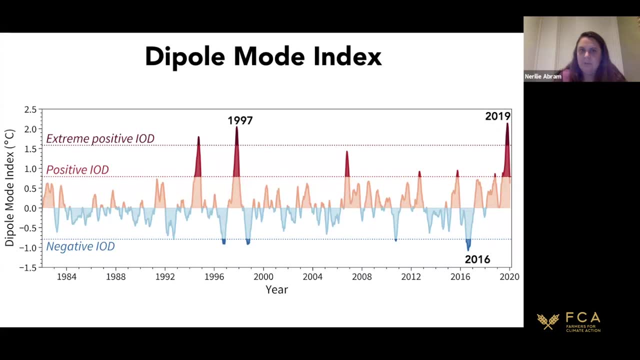 stronger effect on drying Australia and particularly eastern Australia. So this is our observational record of the dipole mode index. So this is where we've got very good observations based on records of sea surface temperature from the east and the west tropical Indian Ocean. So what you can see, 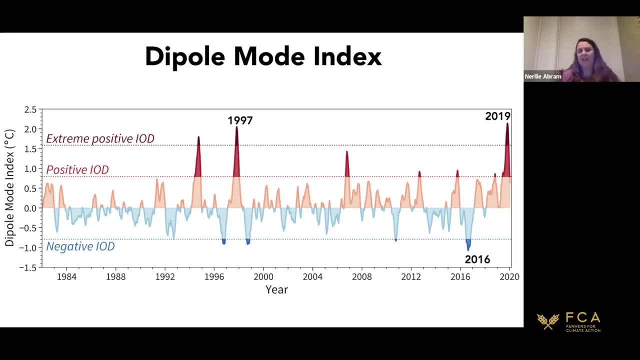 on here in red is where we go into having a positive Indian Ocean dipole event and in dark red is an extreme positive Indian Ocean dipole event. So you can see a couple of spikes in the 1990s. So there was a strong event in 1994, another very large event in 1997.. 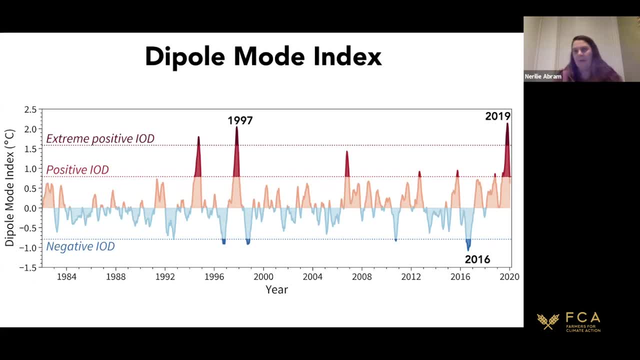 And then you can see 2019 at the end of that time series, And so that's the big event that we had last year, And so something that's quite important I think to point out in here is that the scientific community really only has been working or researching the Indian Ocean dipole. 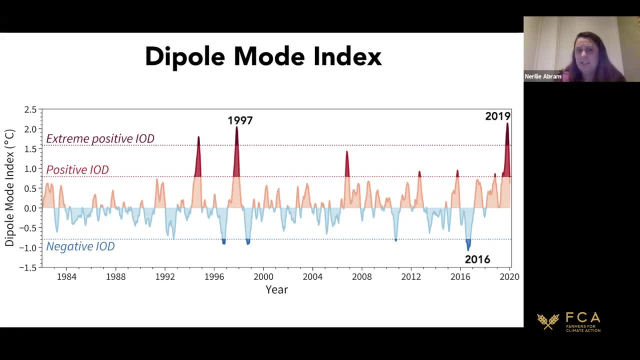 since 1999.. And so that's when it was formally defined and that was following those two big events in 1994 and 1997.. So our understanding of this system is not as good as our understanding for something like the El Niño, where we've been studying that for a few decades longer And also we've 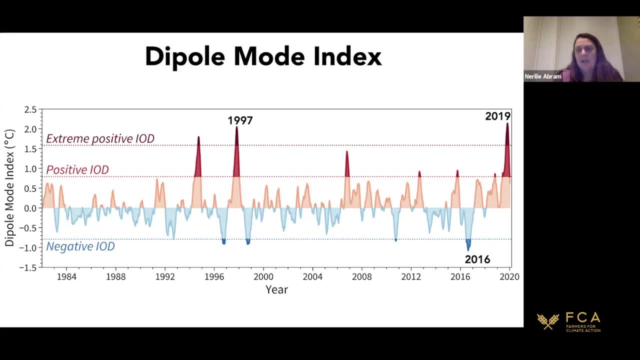 got very few of these big events to be able to study. So 2019, scientifically, that will give us a lot more information to be able to really understand more about the dynamics of this system. So one of the other important things to see with this figure is that when we have these positive 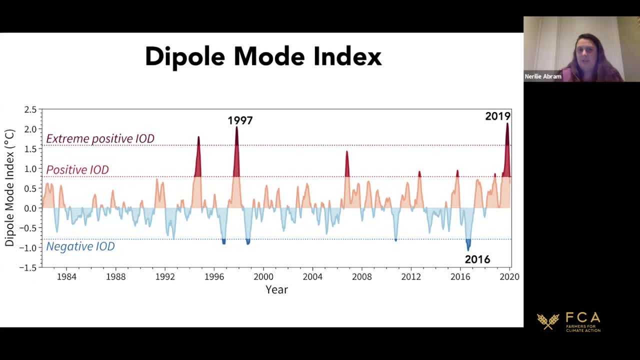 events, they can be very strong, So like 1997, like 2019.. The negative events don't have that same potential. So you can see the strongest event on record here for a negative event is 2016.. But the magnitude of those negative events isn't as strong as the positive events. 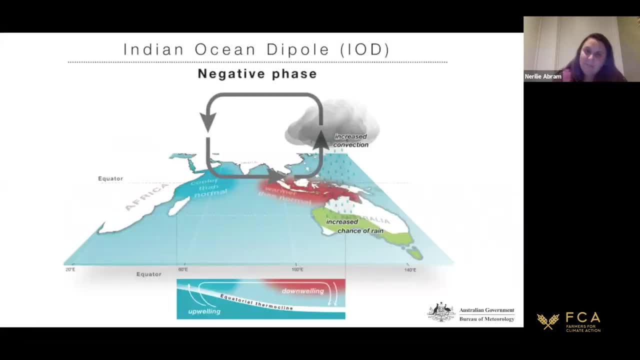 The negative events are still very important, And so in a negative phase we've got warmer than usual water to the northwest of Australia. When we have that warm water we have a lot of evaporation over the ocean, And so then when that air gets drawn down across the 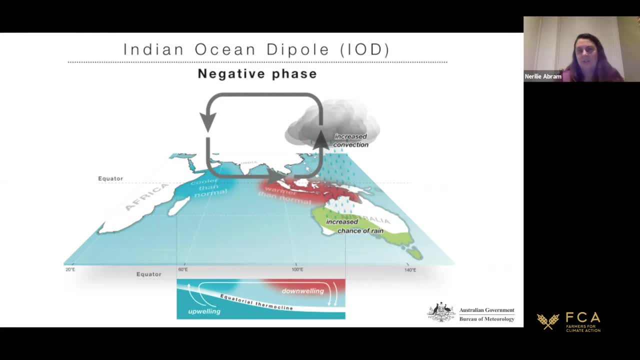 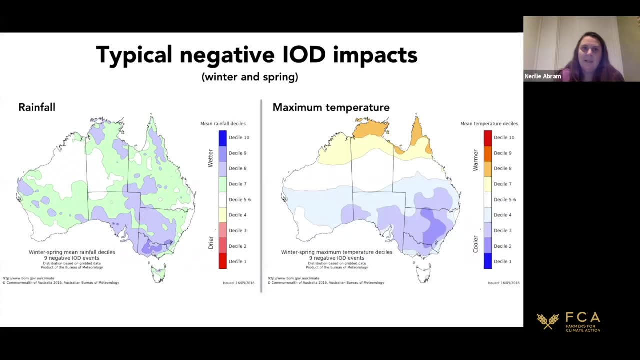 Australia. it's holding a lot of moisture and so you increase the chance of rain. So these are your typical impacts of negative Indian Ocean dipole events. So you can see those wetter conditions across a lot of Australia and particularly down into the southeast. 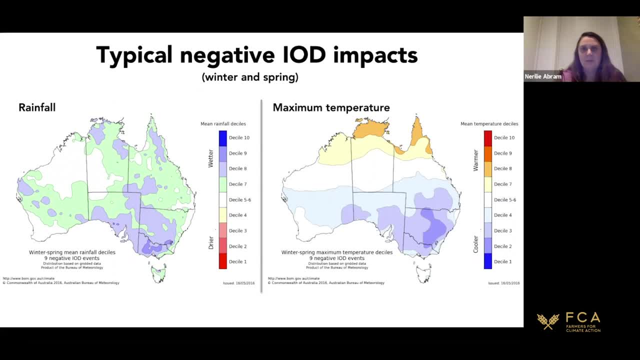 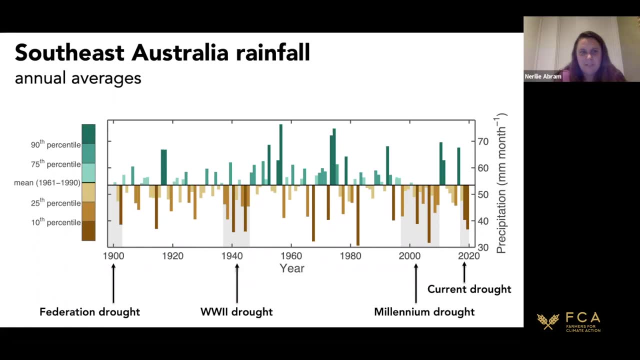 and cooler temperatures as well in the winter and the spring, Right. so the negative events are very important in the Australian context And this is sort of a relatively new way of thinking about the Indian Ocean dipole or, sorry, the Indian Ocean, or actually the effect, the influence of these climate systems on Australia. 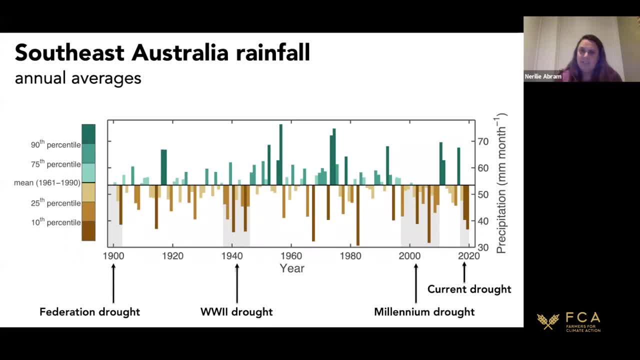 And really sort of pointing to the importance of La Nina events and positive Indian Ocean dipole events. So we have a lot of data on the spatial weather and climate impacts on Australia. So one of the things that's really important in looking at the MEN rainfall bacteria. so you can see here that we've got those two. we've got been given the features of the MEN rainfall. that will be the biggest tool that we can use in breaking drought. So this is a rainfall time series for the southeast of Australia, And so green colours of where we've got above the mean rainfall, Brown colours of where we've got below the main rainfall and that grey shading is showing some of the major droughts that we've had in southeast Australia, including the current drought. 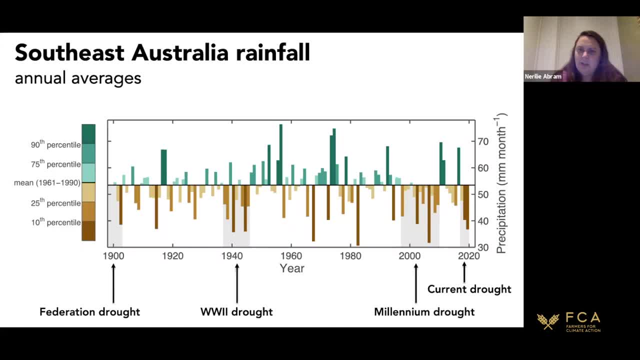 And one of the striking things in this graph is that, of the last 25 or so years in South East Australia, 19 of those have had below average rainfall, And so what's been really unusual in that period of time is the absence of wet years. 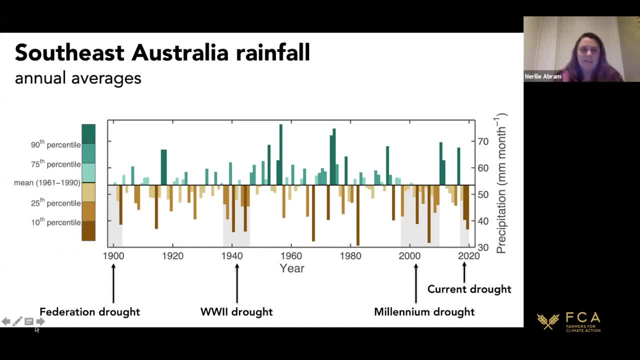 So the only real wet years in this most recent few decades has been the 2010-2011 La Nina event and then the 2016 negative IOD event. So I just wanted to show this, just to show that when we think about these modes of variability, 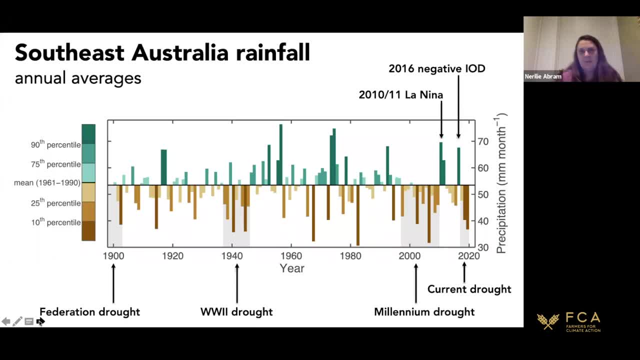 and how they affect Australia. it's not just about the dry conditions that they bring when we have a plow, It's not just a positive Indian Ocean Dipole event or an El Nino event, but also the importance of those opposite phases for breaking those droughts and bringing good rain across the 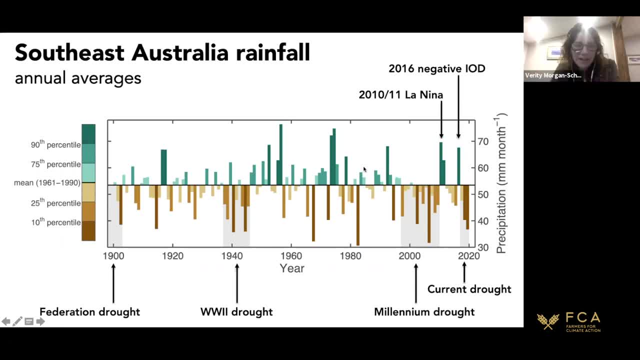 country Nerali. can I ask a question from the chat box? So, Cindy farms near Corrigan in Western Australia. She's just put a question in there in relation to the strong negative IOD events And it's just noted that in 2016,, in particular, Southwest WA had over 20 frost events. 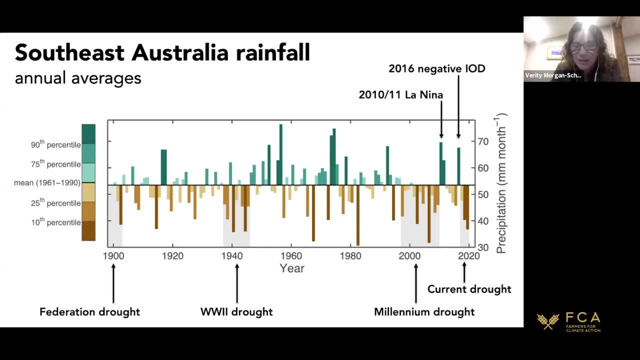 So we talk about the importance of the negative IOD in terms of giving us that opportunity for a little bit more rainfall, But do we know any correlation, or is there one, between the frost events that are occurring? Yeah, so I didn't show the plots here for the minimum temperatures. 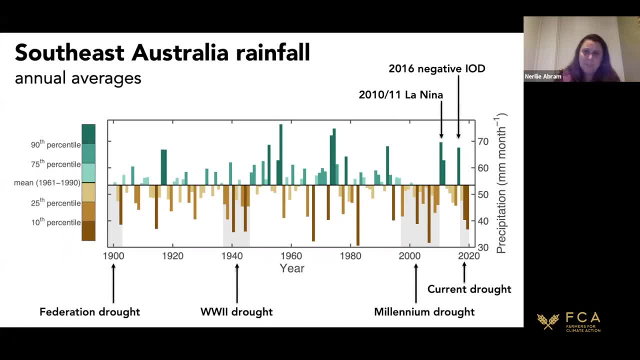 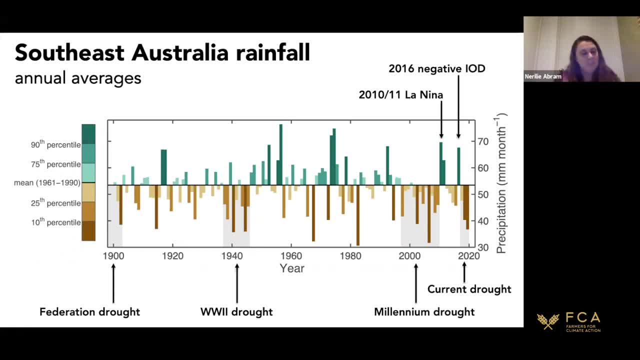 as well, just because of where. well, it's a couple of factors to do with where air masses are coming from, But it also means that if we have a wet environment, then we can take out more heat through evaporation, And so that means that the air doesn't warm up as much as well. 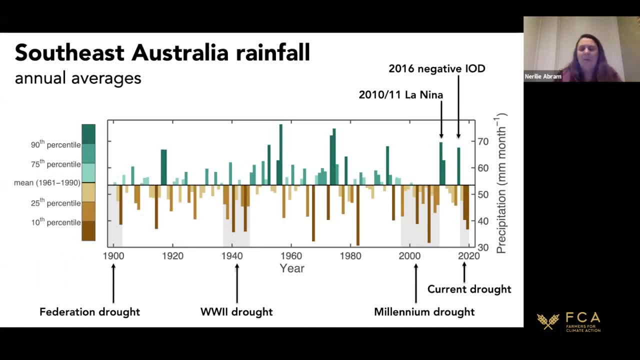 So there is a link, And we have in the past, tended to focus on things like the Indian Ocean Dipole and their effect on rainfall, But they do also have a strong effect on temperature as well. Are you happy with that response? Are there any other questions or do you want me to continue? 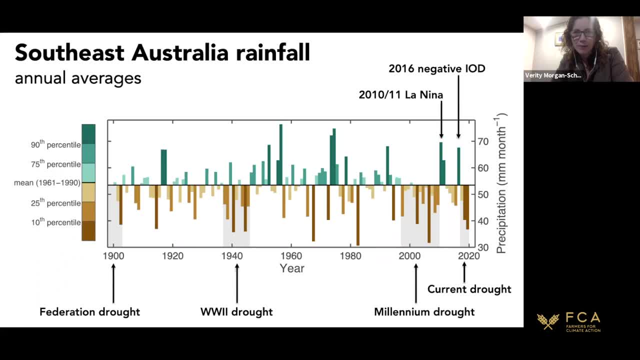 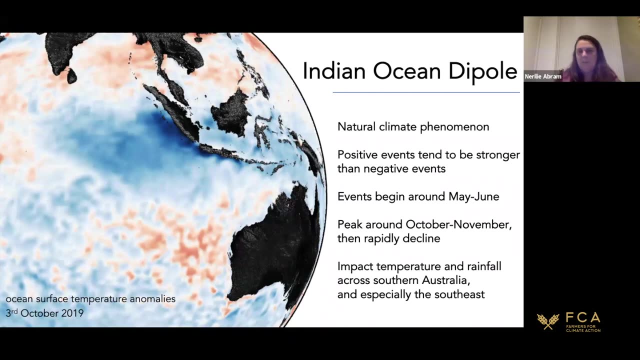 Does anyone want to pop a quick question in or happy to keep going? Yes, Might keep going Nearly. Thank you for addressing that one. Yeah, no problem, Right, So just a summary of the Indian Ocean Dipole. So it is a natural climate phenomenon. 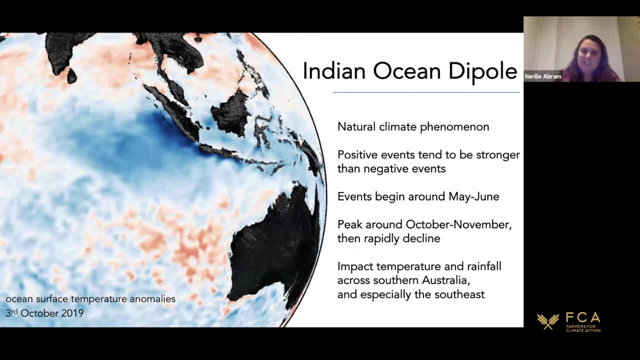 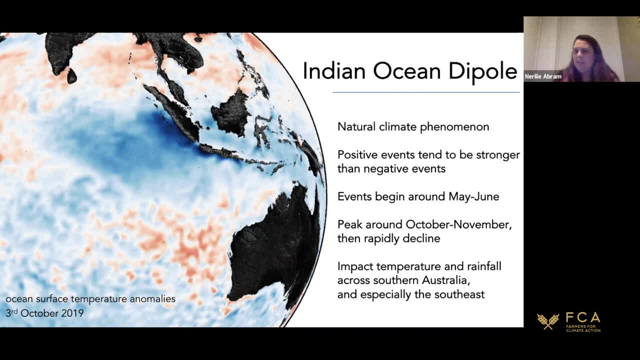 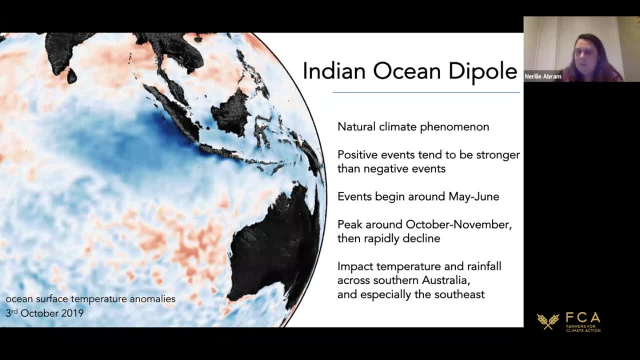 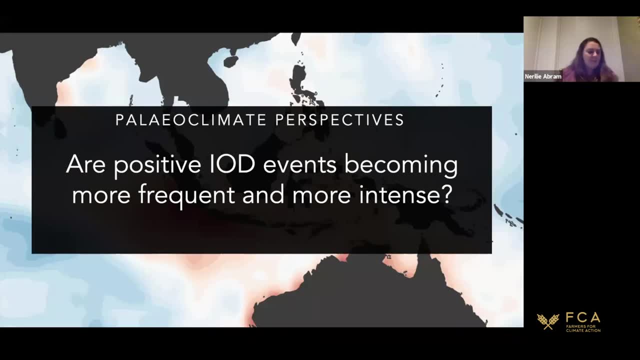 And it impacts temperature and rainfall across southern Australia and particularly in the into the southeast of Australia. Right, so getting on to sort of the research that I've been looking at. So I just wanted to address sort of a couple of the big sort of questions that we were wanting. 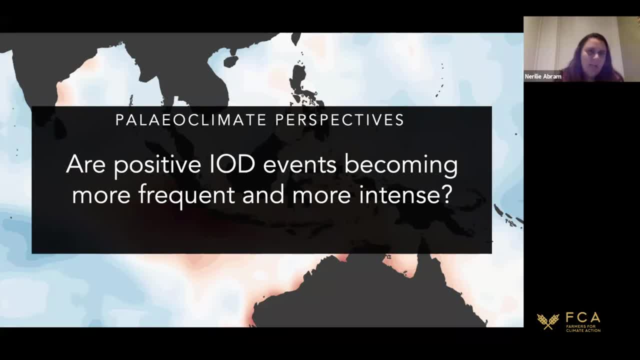 to look at with this. So one of the questions was: are positive Indian Ocean dipolements becoming more frequent and becoming more intense? So this is something that's been suggested based on instrumental data over the 20th century. The problem is that we don't really have good 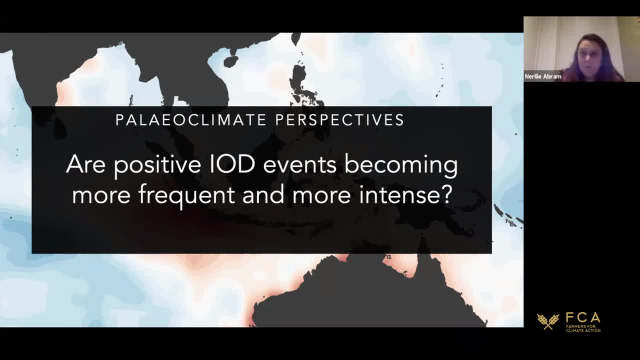 long instrumental records for the Indian Ocean. So we've got very good sea surface temperature data from 1982 onwards. once we've had the satellite monitoring coming into the instrumental record, We think that the sea surface temperature record is reliable back to about 1958 in the Indian Ocean. 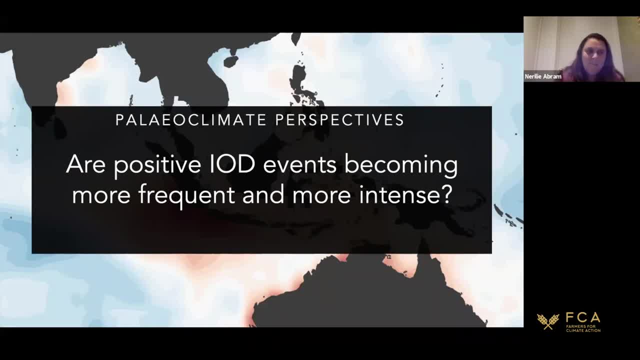 But when we go further back in time than that there's really not a lot of actual measurements that were going into the sea surface temperature products for the Indian Ocean. So that instrumental record suggests that since the 1960s we've had more frequent positive events. 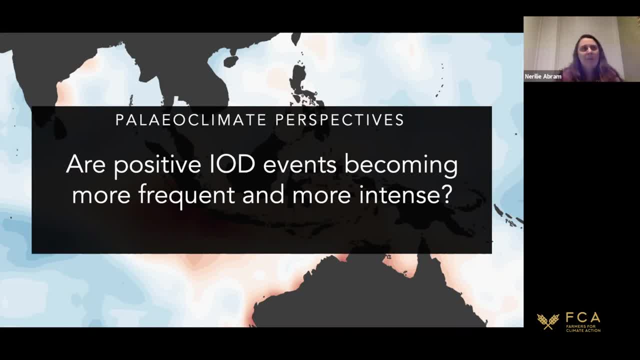 and the events that we've had have become stronger, But we're really not confident In how reliable that instrumental record is before 1960.. The other source of information that we can look at is to go into climate model simulations. And again, when we go and look at climate models, 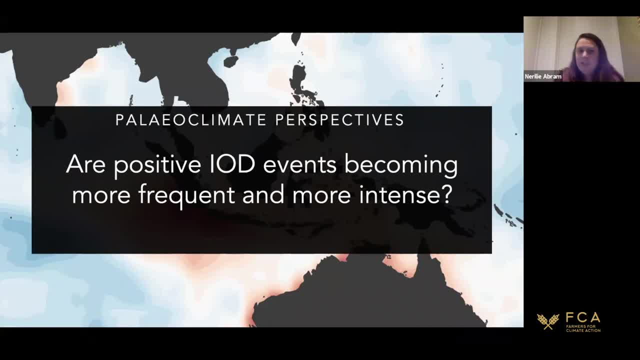 they suggest that you would expect that during the 20th century positive Indian Ocean dipole events should have started to become more frequent because of human caused climate change. But again we've got some pretty serious questions about how much we trust climate models. 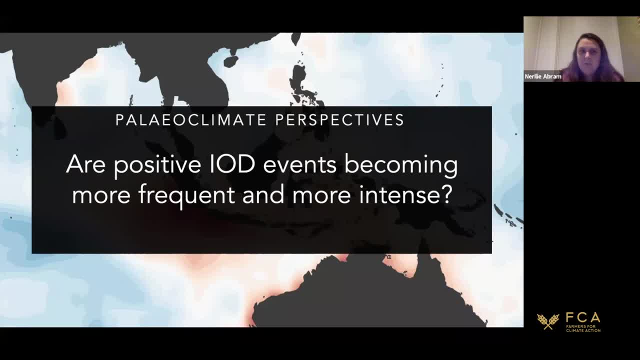 for the Indian Ocean. So there's certain aspects of the Indian Ocean that we know models don't get right, And so how much do we trust that those, what those models are simulating, is correct? And so what we wanted to do here was to bring in another form. 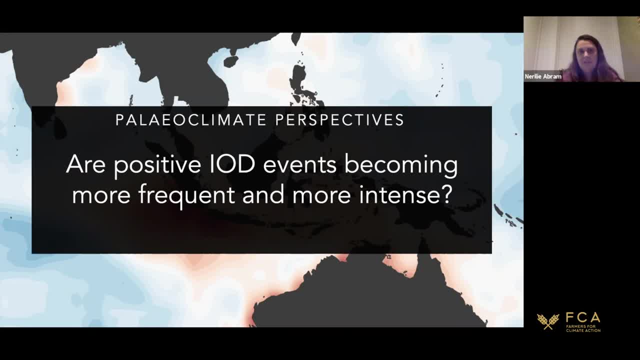 of evidence to see whether that backed up those bits of information that we're getting from the instrumental data And from climate models. if we looked at paleo climate data, did that help to to make it clear whether we could trust those other information sources or not? 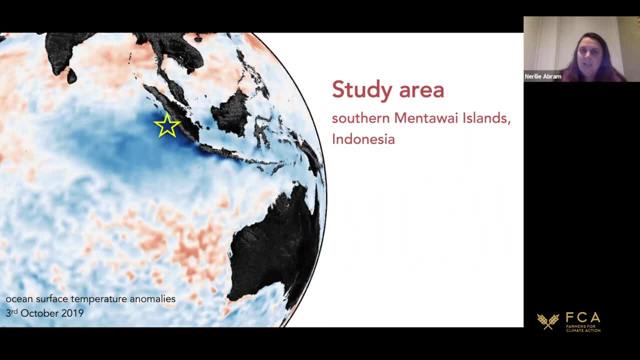 So what we've been doing in this study is to work in this area called the Southern Mentawai Islands. So the Mentawai Islands are a chain of islands around about 100 kilometres offshore of Sumatra in the Eastern Indian Ocean. So it's shown by the map. 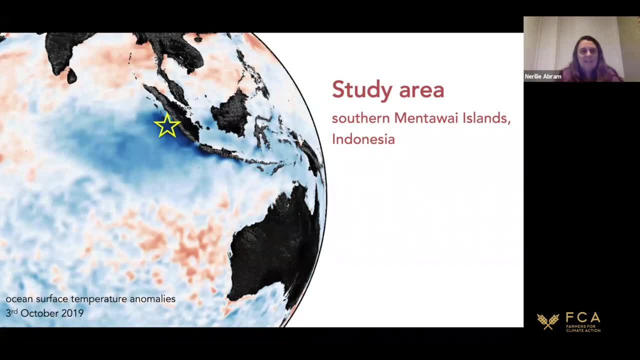 So this star here and the background here, the colours on this map of the ocean surface temperature anomalies for the 3rd of October last year. So what you can see in this image is that when we have one of these positive Indian Ocean dipole events, 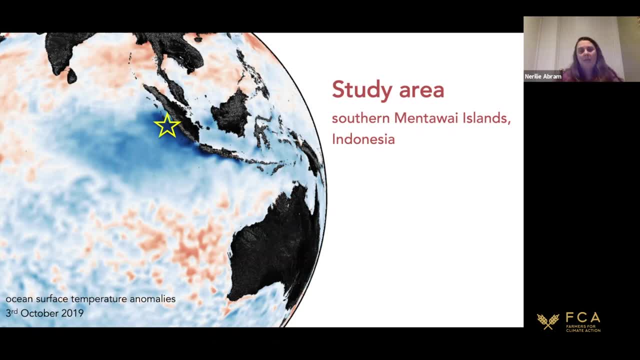 in the Eastern Indian Ocean becomes very cool. This study area is sort of right in the heart of where we see that cooling signal, And what's going on there when we have a positive Indian Ocean dipole event is that we have the winds that run along the coast. 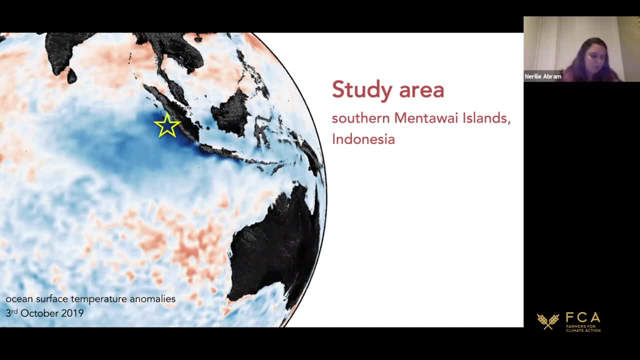 of Java and Sumatra become stronger than usual, the trade winds- And what that does is that it forces the water off the coast of Java and Sumatra to move towards the centre of the Eastern, the centre of the Indian Ocean, and to fill the space that's been left. 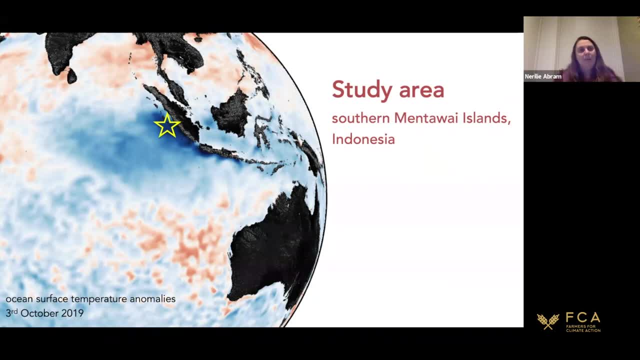 as that water moves towards the centre of the ocean, It pulls up the subsurface water, and that subsurface water is cooler Than the surface of the ocean, And so that's why we get this cool anomaly developing here, And so we chose this study site specifically to be able to look 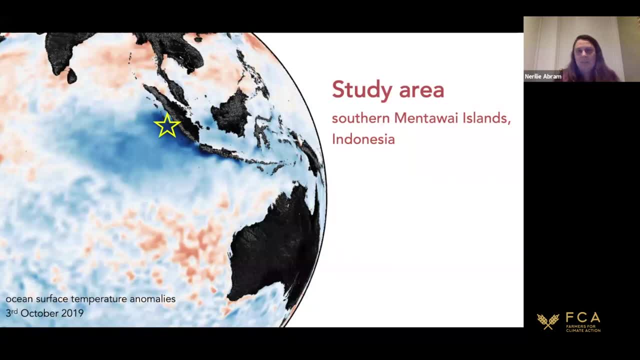 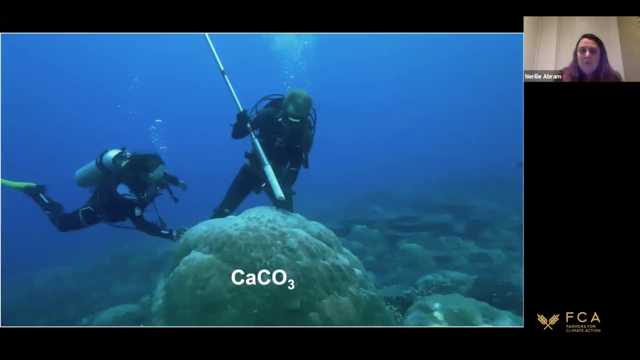 for these characteristic cool ocean temperature anomalies that are associated with the positive phase of the Indian Ocean dipole. So what we were using to go back in time were coral samples. So this is an example of the dipole, The type of work that we do. 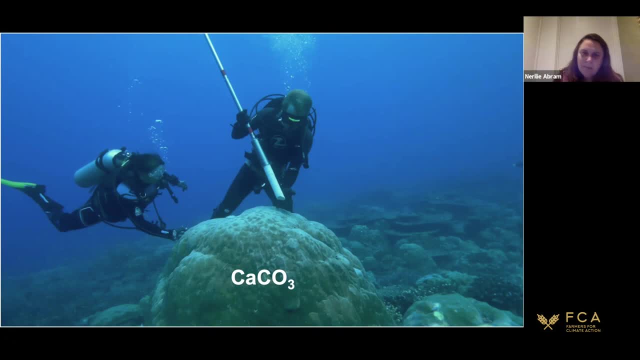 So this is a coral. This is from the Eastern Indian Ocean, from Christmas Island. this particular coral And the type of coral that we use are called parites. They're these very sort of big blocks of coral. They look a little bit like a brown sort of cauliflower underwater. 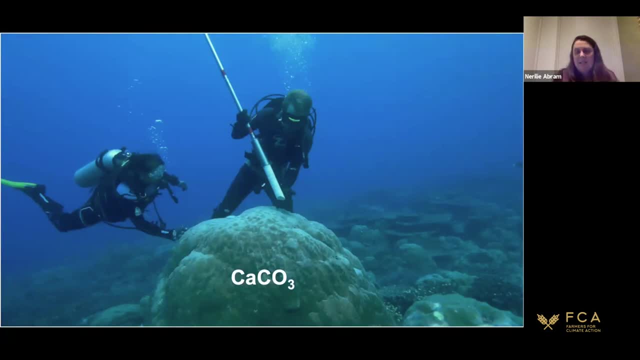 And this sample that you can see here. this coral colony has probably been growing for about 150 years, So every year that this coral is growing in that reef environment it grows around about a centimetre per year And they grow a lot like a tree. 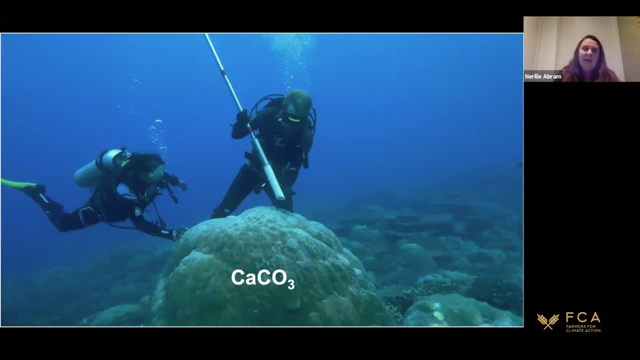 So, as a tree grows, for every year that it's alive, we have a growth ring. The same thing happens with these corals, And so what we can do is to go and drill through that old skeleton. So the coral is only growing. 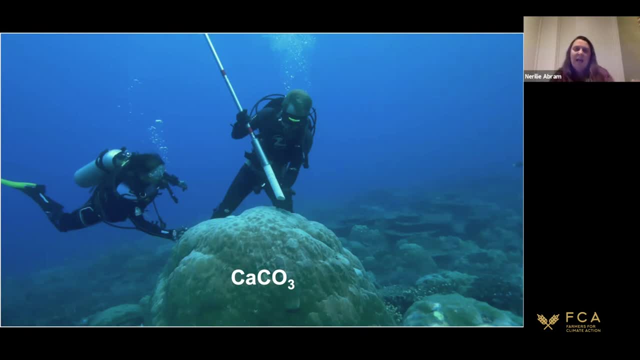 It's only alive on the very outer surface, And so what we do is we go and we drill a core down through one of these corals and go back through those growth bands, And so by doing that, we can build up a record that records the conditions that the coral was growing in. 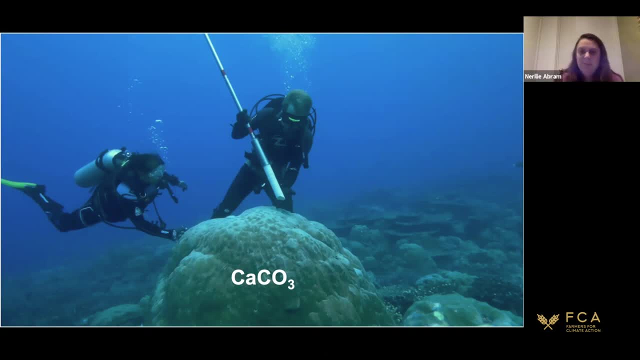 And so these corals, the skeleton, is made out of calcium carbonate. I promise I'm not going to go too much into the chemistry But for people who are interested in this, the main climate measurement or the proxy that we've been using, 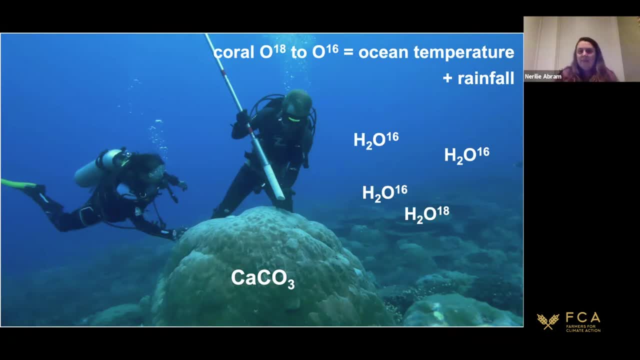 is to look at how heavy those atoms of oxygen are within that calcium carbonate skeleton, And so what we're doing there is we're measuring the ratio of oxygen that weighs has an atomic mass of 18 compared to oxygen that has an atomic mass of 16.. 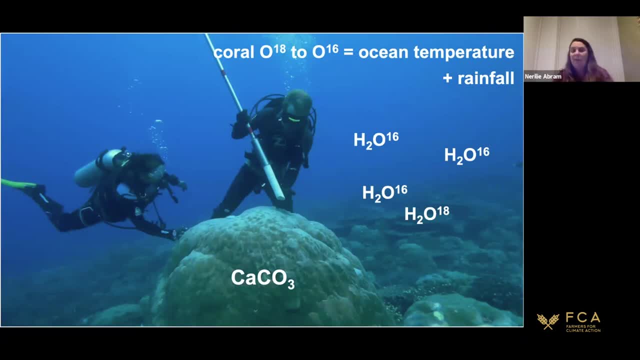 And that varies based on how much oxygen is in the core And that varies based on how much rainfall we're getting over the reef environment. And then the amount of oxygen 18 that the coral takes into its skeleton is directly proportional to the temperature of the ocean. 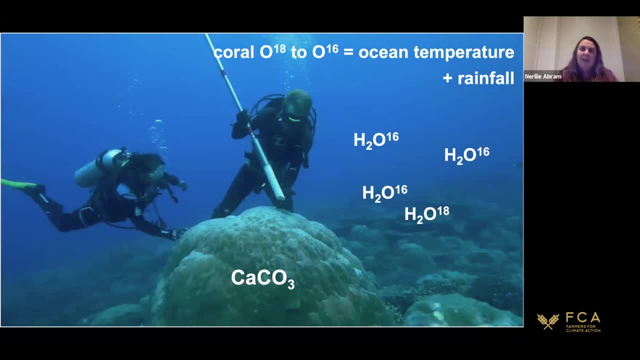 Those things in the tropical ocean go hand in hand. So when we have those cool sea surface temperature anomalies, we also have very dry conditions, And that pushes our oxygen isotope signal in the same direction. So that's what we're doing with these corals. 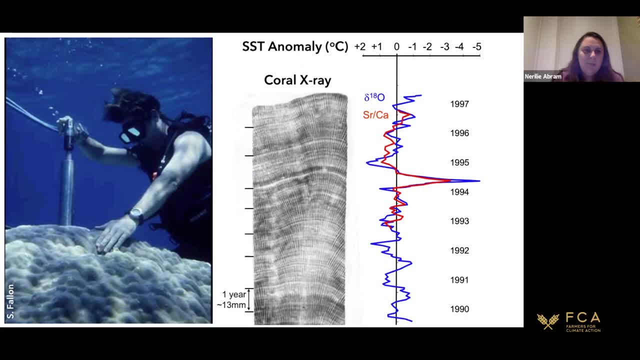 And so here's just another sort of example. So this is again an image of a diver underwater drilling a core through one of these corals. We get that core, we cut a slab of it and we take it just to the local medical center. 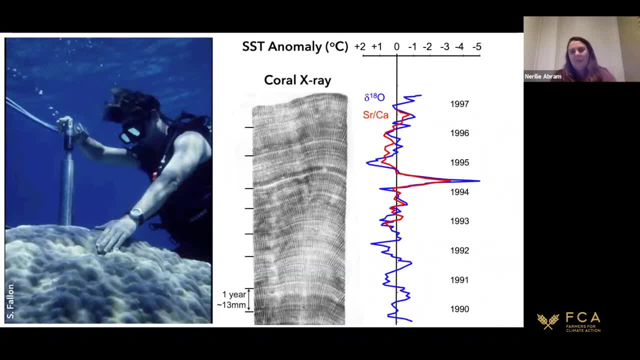 and they take an X-ray of it And we use that to look at the growth banding and then to decide where we want to sample that. We can sample them at really sort of fine detail So we can use that coral to then get a record. 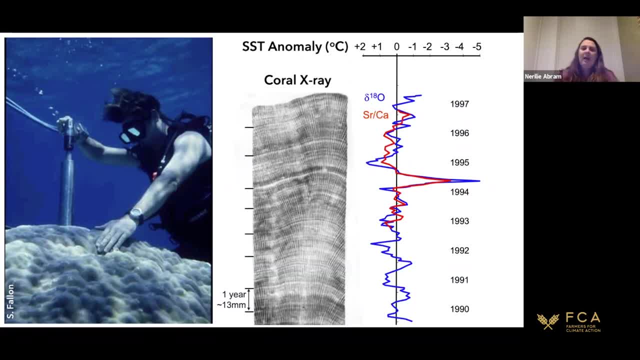 at around about sort of weekly to monthly resolution. looking at the geochemistry This plot here is showing. in blue is the oxygen isotope ratio that we get from this coral And in red is another measurement that we can take, the strontium calcium ratio. 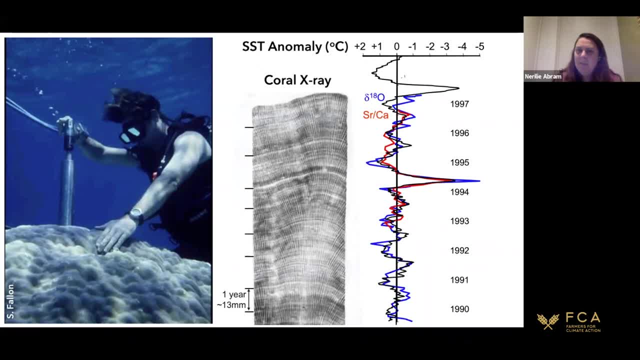 And then, just to plot over to the top black, here now is the instrumental sea surface temperature record from the site where this coral was taken. This is actually a coral from the Mentawai Islands, And so you can see that really big peak in 1994.. 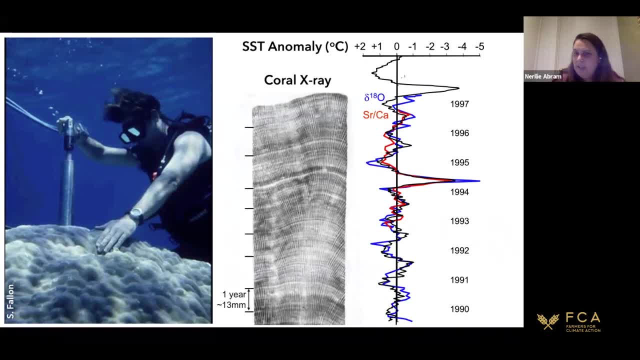 That was the positive Indian Ocean Dipole event in 1994, when we had that really cool temperature off the coast of Sumatra. You can see that. the other one in the instrumental record in 1997.. And this is a coral that died during that 1997 event. 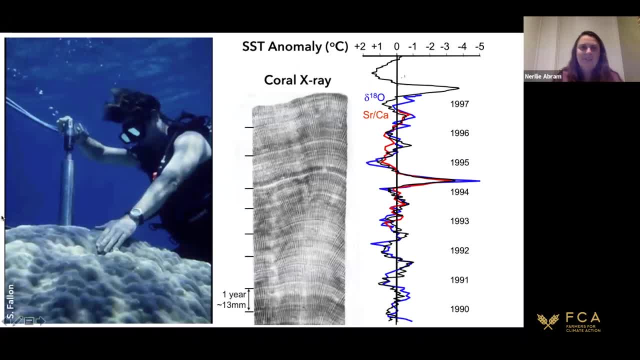 Are there any questions? at this point? I can see a couple of things Nearly. There's one from Rick, who's down near Stanthorpe on the border, And Rick's just put the question that previously we all used to keep an eye on the El Niño-La Niña dynamic. 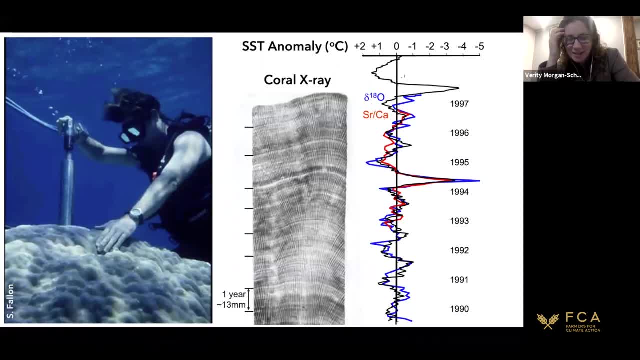 as an insight into the next season. Is it the case now that the IOD is more dominant and therefore a better indicator for farmers to be keeping an eye on? And I know Pete Thompson up at ROMA has also put a comment around the IOD being a better indicator than the SOI- 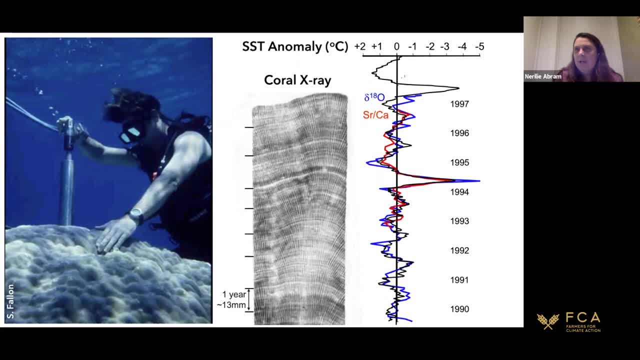 I think that that partly depends on where you are. So if you are in Queensland, then probably the El Niño is going to be more of an influence for you than the Indian Ocean Dipole. If you're in the South West, the South East of Australia, 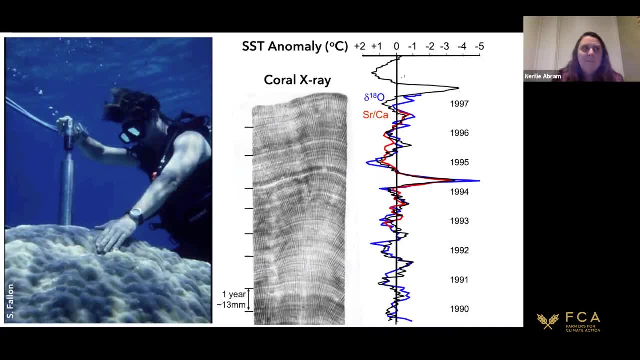 so parts of New South Wales and Victoria, then you really do have an interaction there between the Indian Ocean Dipole. You've also got what's happening in the Pacific, but you've also then got what's happening in the Southern Ocean as well with the Southern Annular Mode. 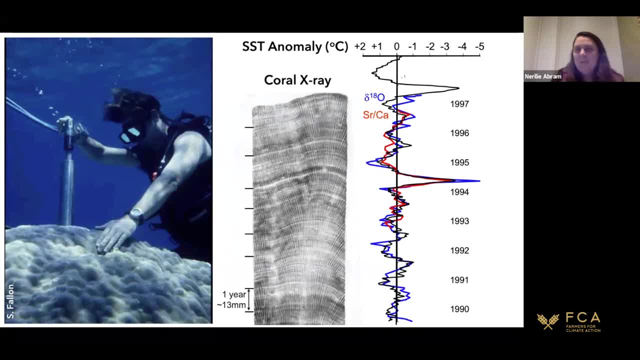 So that's one of the reasons why I guess, when we have questions about why have we had a drought in South Eastern Australia, it's not. It's not necessarily a simple question to answer, because we've got so many different factors that play into the climate in that part of Australia. 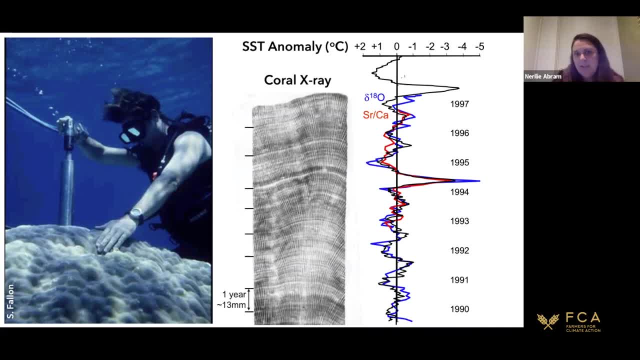 And so we can have, for example, the drought that we've had since 2017. looks like probably what we were looking at is a succession of different climate features, which meant that we had this run of a number of years where we didn't have good rates. 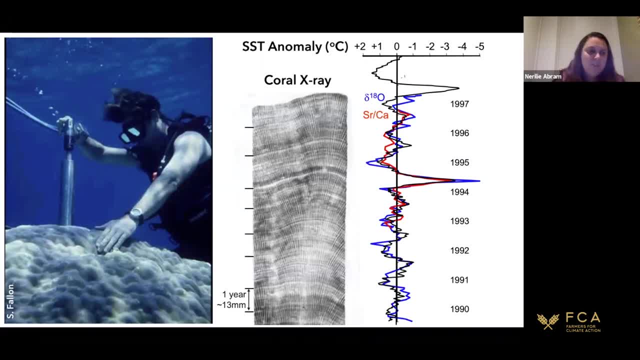 And so that was really meaningful with 2019, the Indian Ocean Dipole being one of the factors that was playing out then. So yeah, so the question is. The answer to the question is quite nuanced. It depends on where you are. 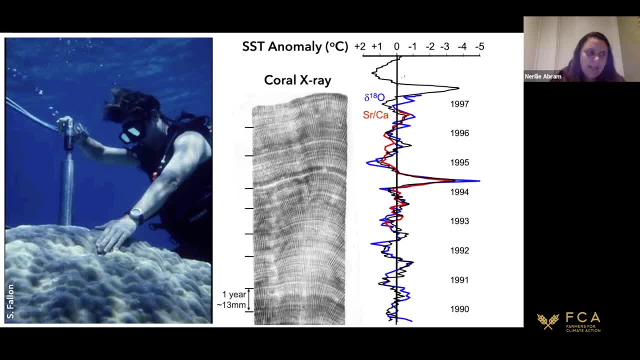 But I think one thing that we are seeing is that probably the Indian Ocean has more of an influence than what we previously realised And that's partly because we've had so few of these big events to really sort of study And we've been studying this climate feature for a lot less. 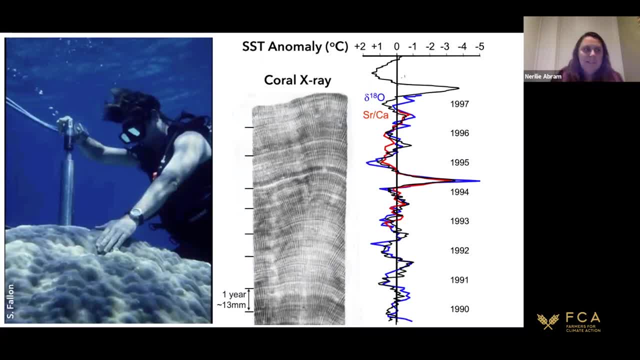 But it is something that the Bureau does include as part of their climate drivers, that they're really monitoring because they know that it has an effect. And Neralee. there's another question from Steve Hobbs, who farms Stanley Caniva in Victoria. 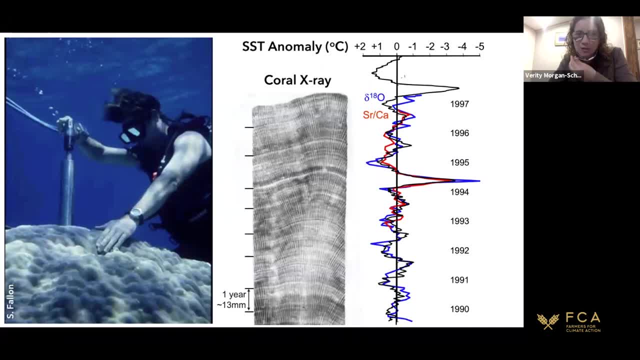 And Steve sort of made a comment, but it's really caught my interest. The point that he's made is that the worst droughts that he's experienced in that region are a combination of a negative IOD and an El Niño year. 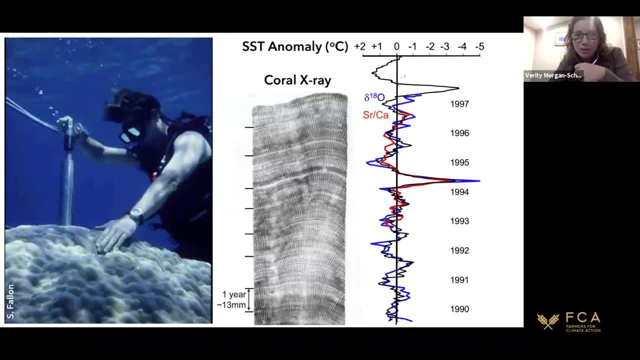 And he's also noted that these also coincide with very low ozone concentrations. Are you able to, I guess, provide comment on- Oops, sorry about the dog on Steve's question, So a negative IOD? I guess we would expect that to sort of have a wetter condition. 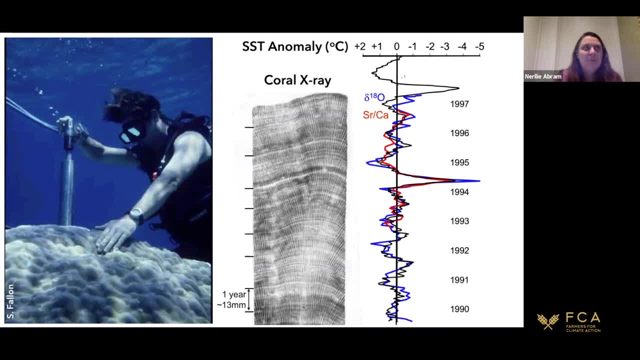 So, and I guess noting as well that the negative events tend to be a lot weaker than the positive events. So in that situation probably yes, that's where El Niño events have been sort of more important, And the ozone one is interesting. 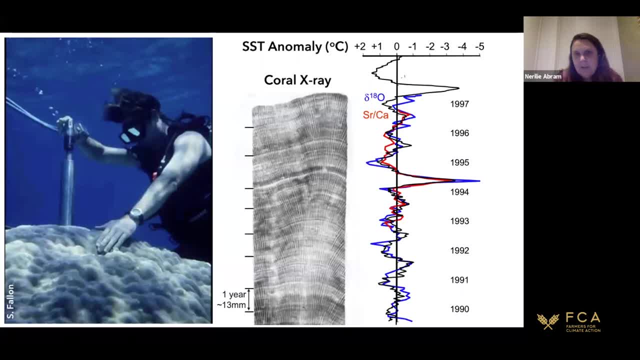 And I guess that's another interesting thing that we saw play out in 2017, was that we had quite a We had quite a rare event over Antarctica, where the polar vortex in the springtime broke down very quickly, And so what that does is that it pushes the southern annular mode. 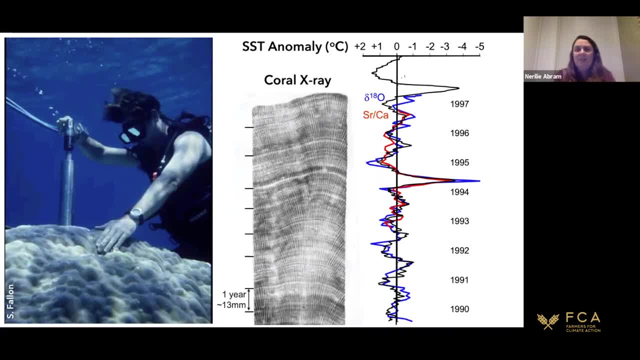 into a negative phase which moves the southern hemisphere westerlies further north, And so that was one of the major influences that we saw in northern New South Wales last year to the bushfire risk as well, where we saw a lot of frontal activity coming across Australia. So a lot of those cold fronts were ahead of the fronts. They were drawing hot and dry air from across Australia towards the east coast And then the fronts coming through and not having any rain because that air that was being drawn into them was so dry. 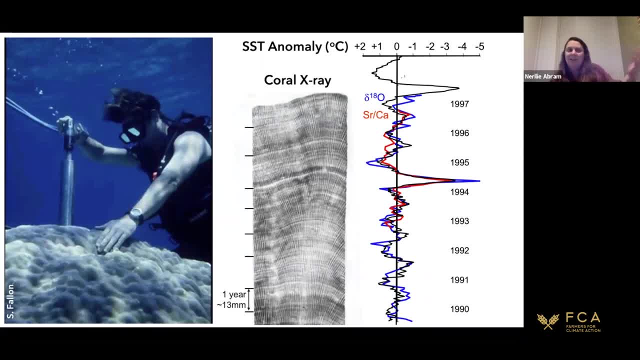 So that was where we saw an interaction between what was going on in the Indian Ocean and also what was happening in Antarctica. So I'm not sure if that was a great answer to that question. Yes, Steve, did you want to comment? 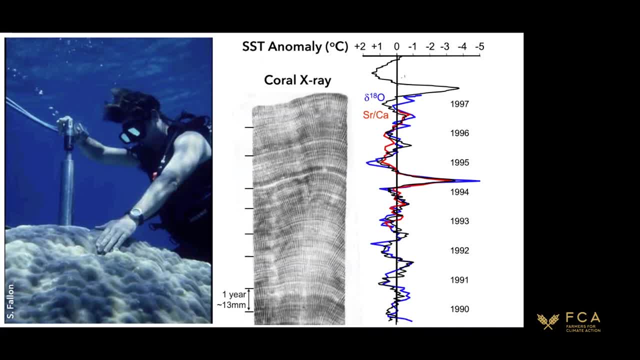 Yes, please. Thank you. None of the data I've seen so far I'm on the Darling Downs of Queensland. None of the data that I've seen so far suggests that it's got a significant impact here, And in fact I would argue that. 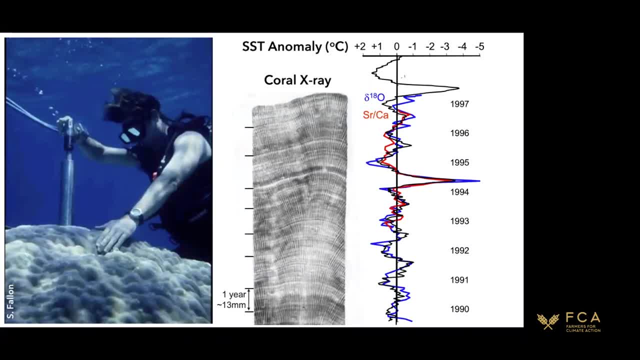 it really overpowers ENSO here, The only real rain we've had from the Indian Ocean, And basically we've lost that rainfall in the last 10 or 15 years anyhow, And I think the mechanism has something to do with Asian aerosols. 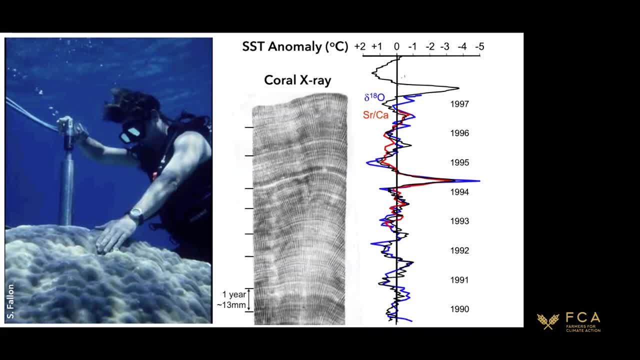 Most of the rain falls in the Pilbara and down the Tanami before it gets to us, And that's why we've got a lot less winter cropping on the Darling Downs, because we're just not getting the rain through the. Yeah, But- and I'd just like you to confirm or deny my perception there- 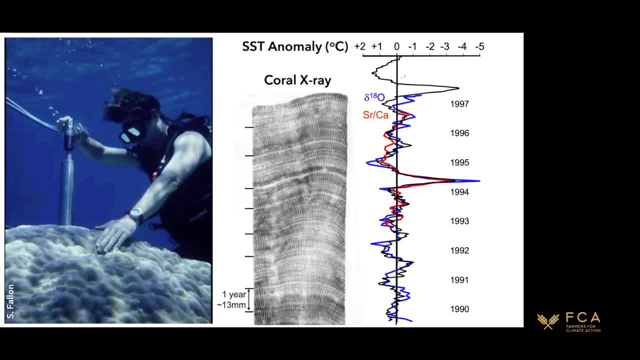 but I don't really see it- having watched it for 40 or 50 years- as a significant thing to change over to using where I am. I don't, And I would argue that ENSO is much more powerful in this situation here. 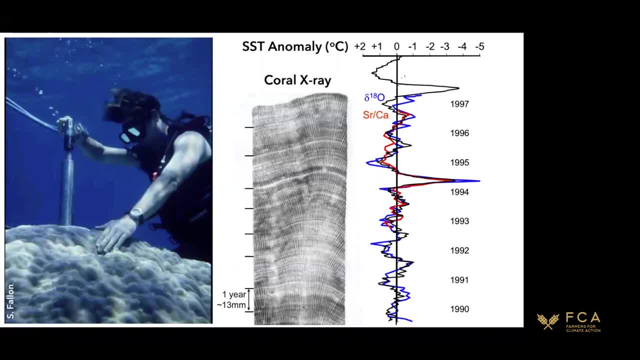 You might be aware that ENSO is quite a significant thing where if you've got to start the water, you're not a lot of water use going on up to the Perth or the Inverness川 or the Eifsjord Islands. and you're so quickly getting more rain there and more care for your people. you're getting more drought coverage And that's when that is going to get to us and we'll see them in some of the Signals. a little about Charleville. And then, by the time, Birdsville's big droughts are typically when it's neither El Niño or La Niño, for example, Whereas for the rest of us- and El Niño certainly dries it out for us. Yeah, I can leave it at that, if you'd like. 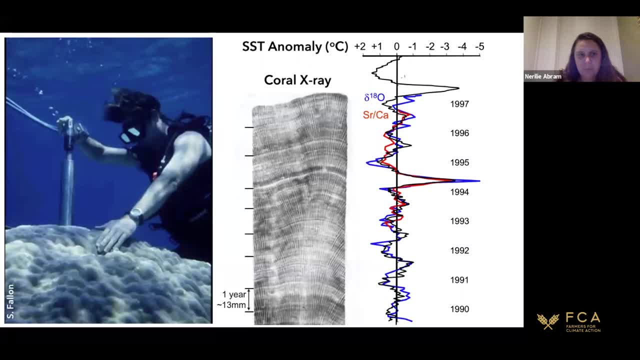 Yeah, no, I would just confirm, Yeah, your intuition there in that, yeah, El Nino is definitely sort of more of an influence than the Indian Ocean Dipole. So what we see for the Indian Ocean Dipole is that the rainfall that comes across Australia tends to come through in these northwest cloud bands, And so you can see those on the satellite map sometimes, when these are active, that you have sort of these bands of cloud that stretch from sort of the Kimberley area all the way down towards Victoria. 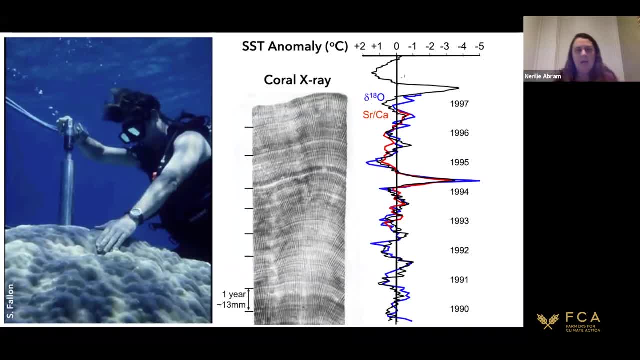 And so that's the area where you really have a strong rainfall impact And so that sort of northwest pattern doesn't tend to sort of push into Queensland as much. Yes, thank you, And I know the Pilbara rainfall has been increasing for 20 years or so. Have a look at Patchar, for example. It used to have a long term median of two inches and it's been quite a bit higher ever since, probably 15 years, 10 or 15 years. 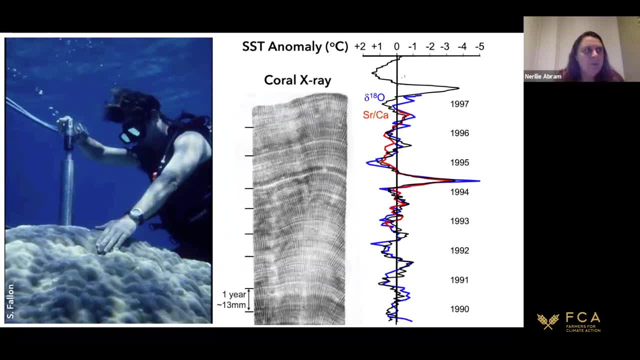 Yeah, There are some different things going on there as well. So when we start to look at the northern parts of Australia, we start to be getting into some summer dominated rainfall, And so the Indian Ocean Dipole really isn't a dominant influence in those seasons. 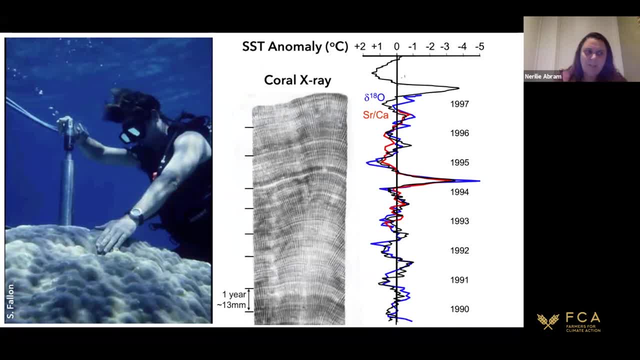 So it tends to have its strongest impact in the winter and spring, And so we see that across the southern parts of Australia where you have sort of more winter dominated rainfall. Yeah, thank you. And the only other comment I'd just like to make: I see ENSO as being an Indian Ocean Pacification event. really, They're both involved rather than just the Pacific. 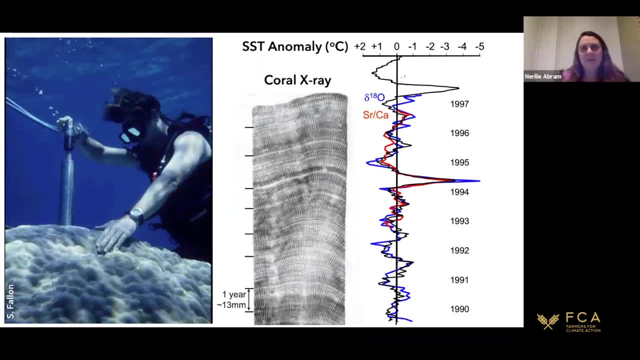 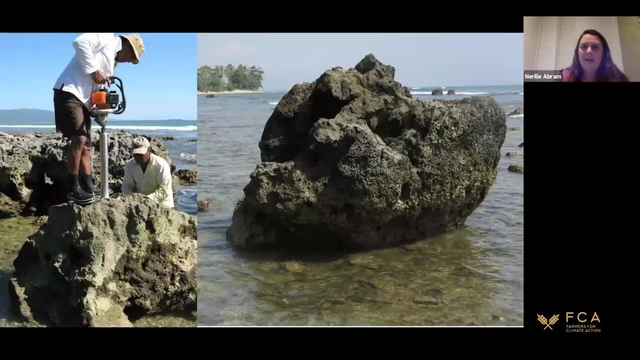 Yeah, definitely, And that's something that our research has shown as well is that they are quite closely linked. Cool, So I'll keep on going and actually get on to some of the results that we've got. So I showed some pictures before. 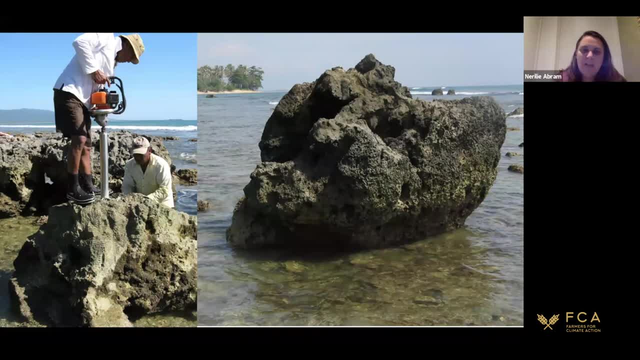 So these are four of the type of work that we've done using underwater corals, So they're corals that are living on the reef at the time, And so we can go back sort of 150, 200 years using those types of corals. To go back further in time, we have to start. 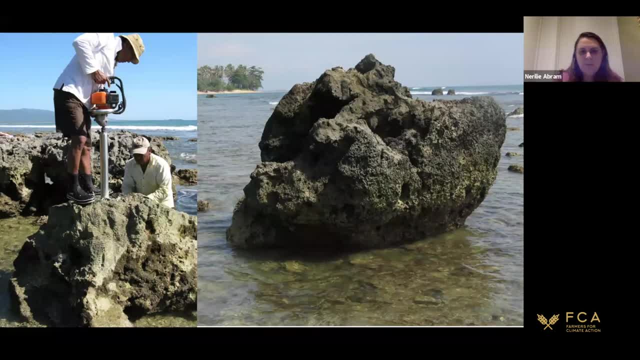 looking at fossil corals, And so these are a couple of examples of fossil corals we've drilled in Indonesia. In Indonesia, of course, there's a lot of earthquakes and tsunamis, And what that does is that it rips up. 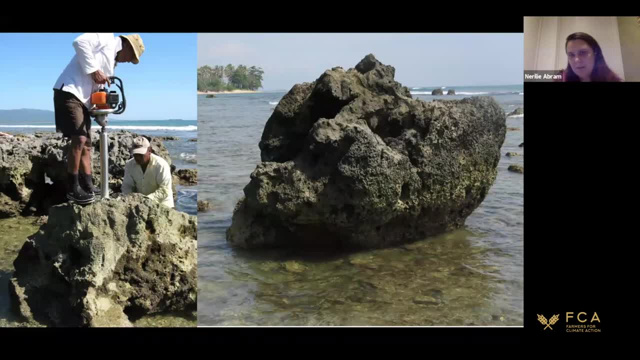 corals that are growing in the reef environment and sort of throws them up onto beaches or takes the entire reef and moves it up above sea level, And so around the coast of Indonesia we can find fossil corals of all sorts of ages, And so those are the types of samples that we've been using in this study to go further back in time in reconstructing the Indian Ocean Dipole. 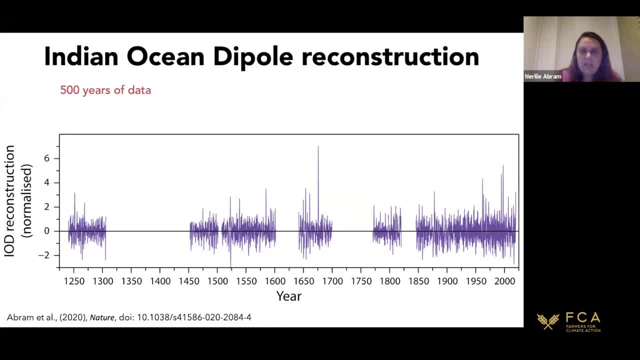 So this is the reconstruction that we have so far. So this is work that was published just a few weeks ago in Nature. This blue line, blue squiggly line- probably doesn't mean much to anyone just looking at it, but this is just showing the data that we've got. You can see there are gaps in the data and that's. 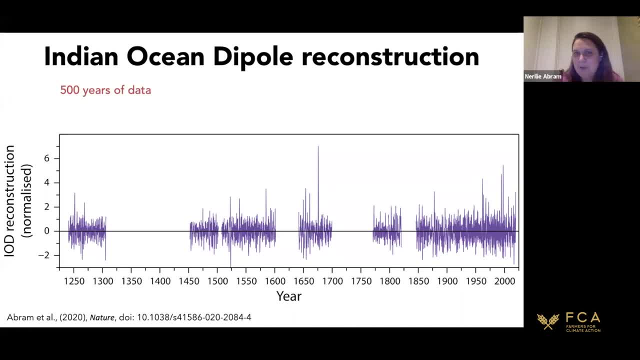 just showing periods of time where we haven't found those fossil corals yet of the right age to be able to fill those gaps. But we do have, across this data, 500 years of Indian Ocean Dipole data, now based on our coral reconstructions from off the coast of Sumatra. 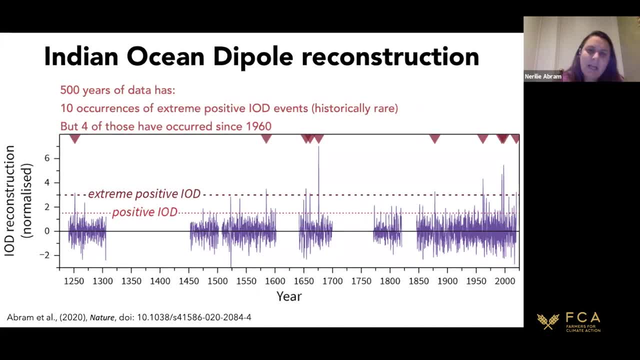 So so a bit of interpretation on this, So we can go through this record and we can see when the reconstruction is exceeding those thresholds. that would indicate that we've got a positive Indian Ocean Dipole event or an extreme positive Indian Ocean Dipole event. 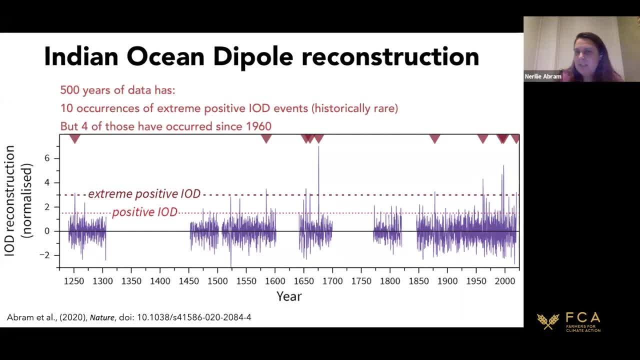 And so what we can see is that extreme events like what we saw in 2019, have historically been very rare. So, across 500 years of data, we only detect 10 occurrences of those events. But what we can also see is that four of those events have occurred since the 1960s. So when we look at that instrumental record and we and we see that it seems since the 1960s that there has been 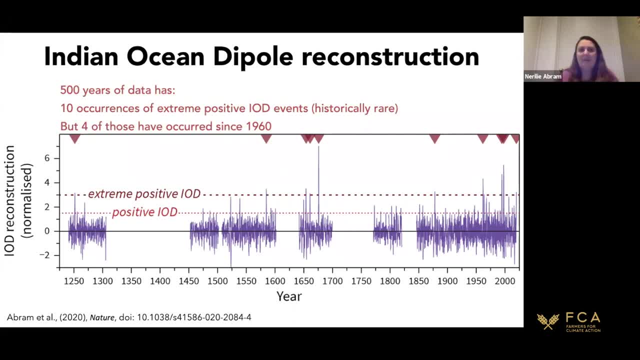 these events have been unusually common. When we look across 500 years of data, we also get that same picture: that these are have been rare events, but they appear to be becoming more common now. So we can- we can- look at that in a different way. So this is where we 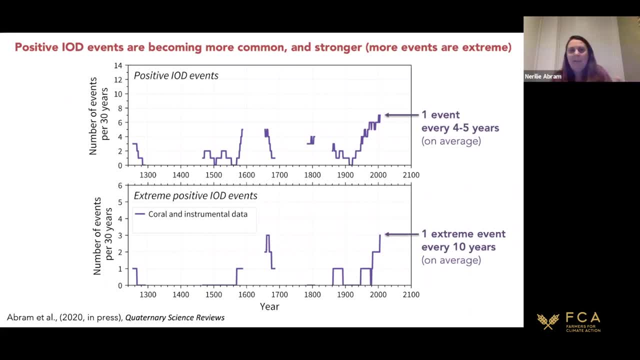 take 30 year windows of that data and we count up how many of these positive events, or how many of those extreme positive events, have we had in each of those 30 year windows, And so what you can see is a natural variability and natural fluctuation of these events. 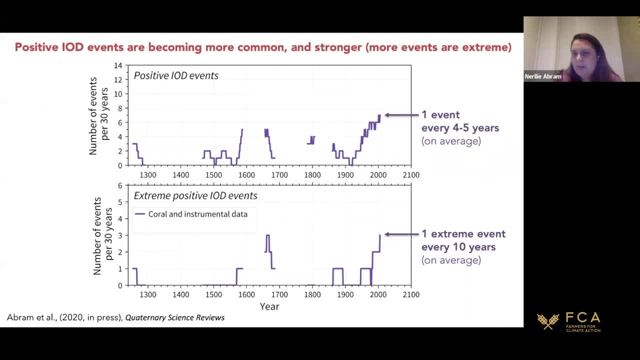 And then we can see in the most recent part of the record that we're now either at a level for positive events, where we've got the most frequent events of any time in what we've reconstructed over the last millennium, and for extreme positive events we're 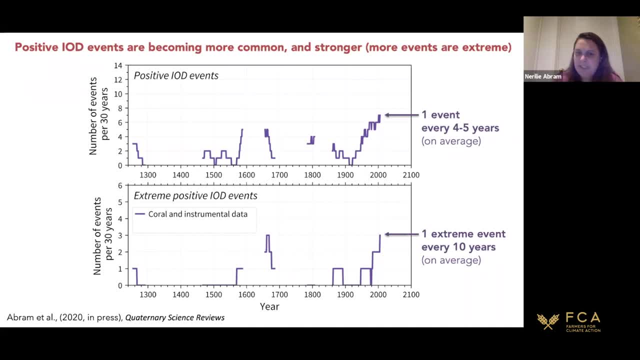 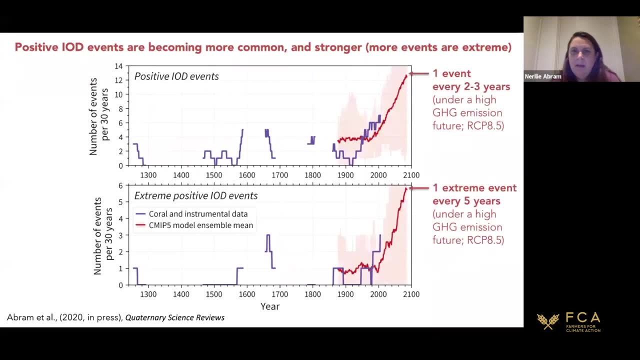 at a level that's equivalent to the highest that we've seen in the past 1000 years, or that 500 years of data that we have for the last millennium Right And so. so what we can do, then, is to compare that with what we see from climate model simulations, both for the historical period. 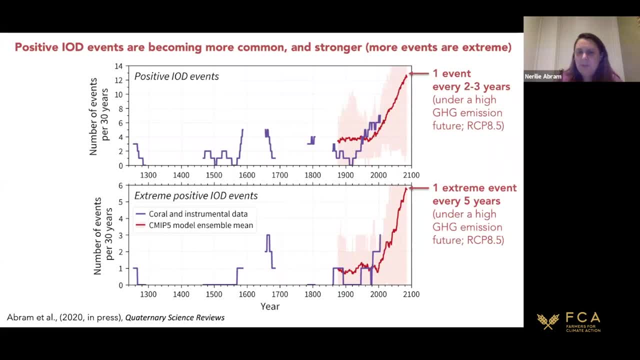 but also then looking forward if we run those climate models into the future, In this case using a high greenhouse gas emissions scenario, So scientifically we refer to that as an RCP 8.5 scenario. It doesn't matter if that doesn't mean anything to you, but this is. 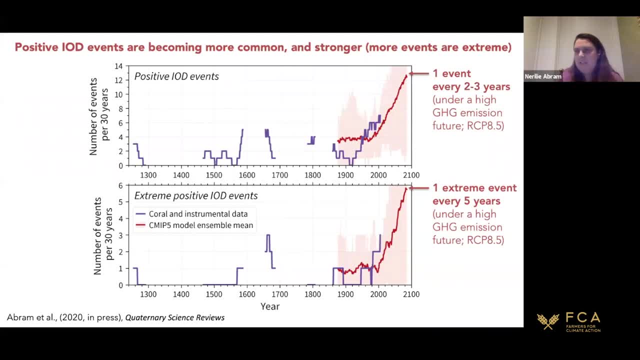 this is our sort of high end If we don't do anything to reduce greenhouse gas emissions. this is the trajectory that we're on, And so what we what you can see is, across our coral data, our instrumental data and our climate models, we start to have this consistent picture that we're seeing an increase in positive events. we're seeing more of the extreme events, and that's a trajectory that we expect to continue. 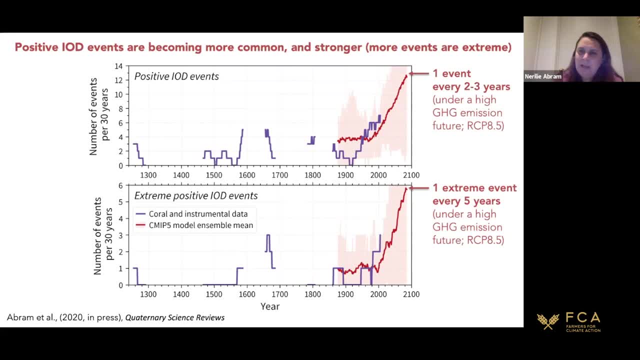 with human caused climate change under a high greenhouse gas emission future, And so by the end of the century, if we continue on this high pathway, the average of these climate models would be suggesting that we'd be expecting to see positive events happening roughly one every two to three years, and that we would expect to have an extreme event roughly once every five years of those positive events that we're having. 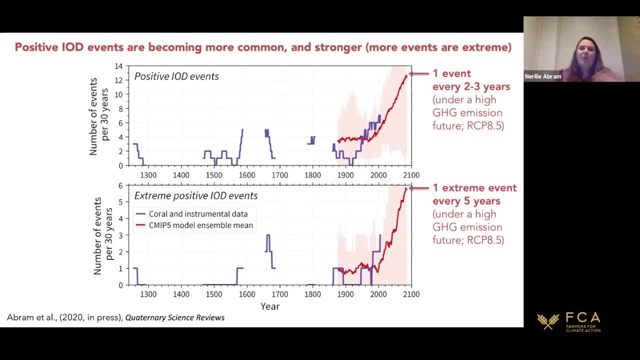 So that's kind of the where we can now look at what's our range of natural variability, And when we combine all that together, we can see that we are changing the system and we are moving it into an area that we haven't experienced before. 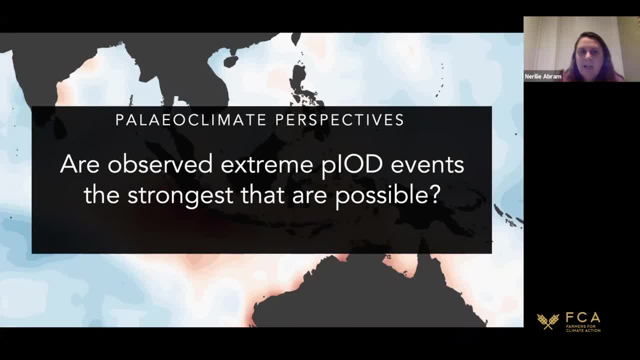 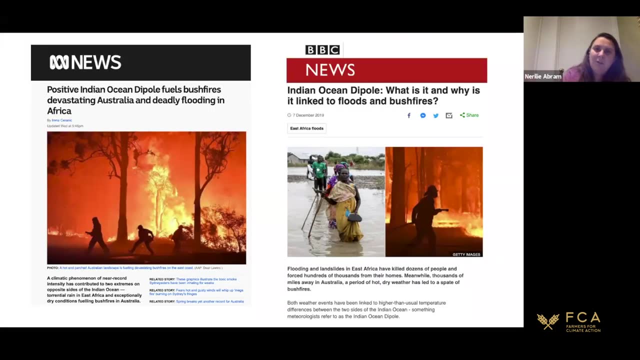 So one of the other questions that we wanted to ask were the most extreme events that we've experienced in recent decades. so events like 1997 and 2019, are they the strongest events that are possible? And so obviously, 2019, there were major impacts of that, particularly in southeastern Australia, with the bushfires that we saw. that came along after the very dry and hot conditions. 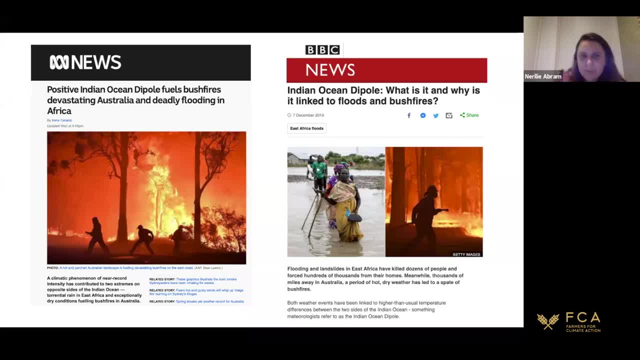 There has been work to say that in Victoria the worst bushfire season that we've seen in the last year or so has been the most extreme event that we've seen in the last year or so, and that we tend to follow times when you've had a positive Indian Ocean Dipole event And then we've also got the impacts that we see in Africa as well, where they've had very heavy rains and then faced locust plagues associated with those very heavy rains. 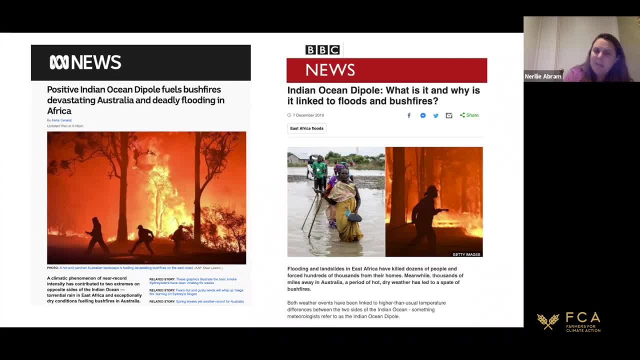 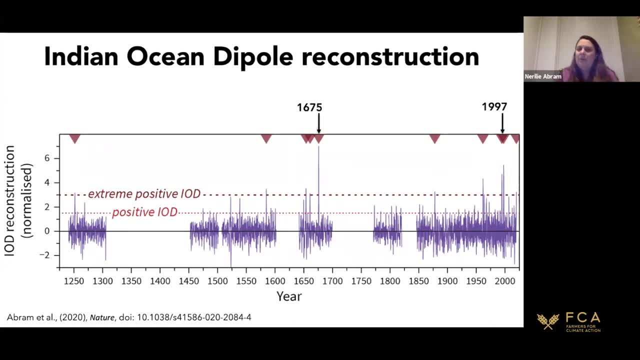 So these events can have some very extreme impacts, So important to take a look at whether our short instrumental record tells us what is possible. And so what I wanted to point out here is just to highlight- you can see here- the magnitude of 1997 events in our reconstruction compared to this one event that we reconstructed in 1675, which is much larger. So if we go and zoom in, 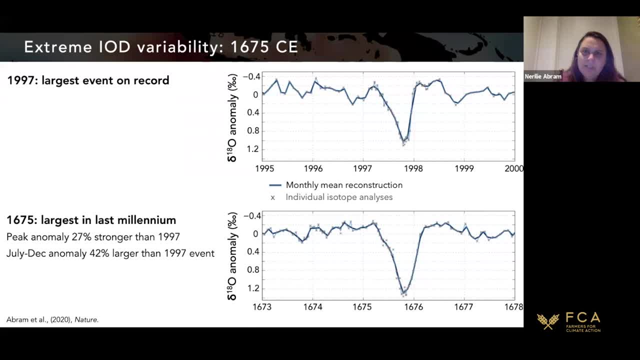 to the detail that we reconstruct from the corals. you can see the 1997 event at the top there, And then 1675, which is the largest event that we've reconstructed in the last millennium, And so the peak anomaly of this event suggests that it was. 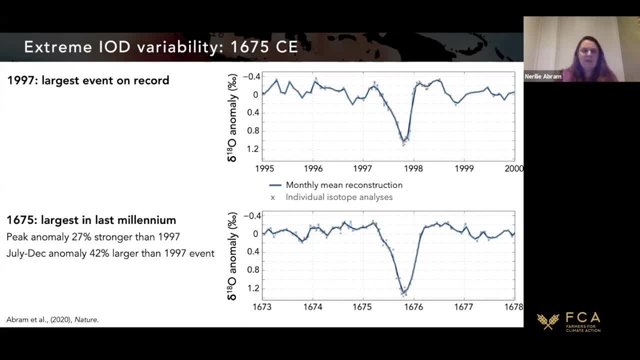 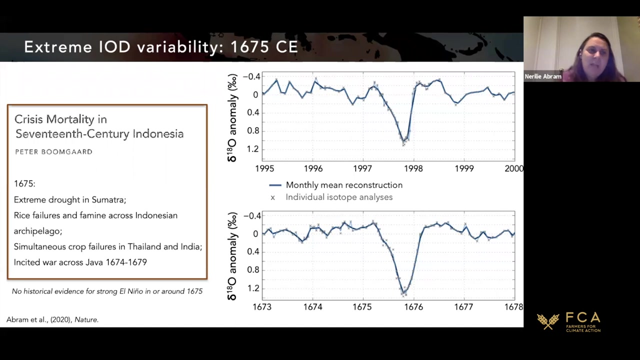 around about 30% stronger to about 40% stronger than 1997, if you take the average across that full July to December interval. So we don't have historical records from Australia to be able to see what sort of impact did this have. We would expect that it would have had a major impact, but we do have information that we can find in historical documents from Indonesia and other parts of Asia. 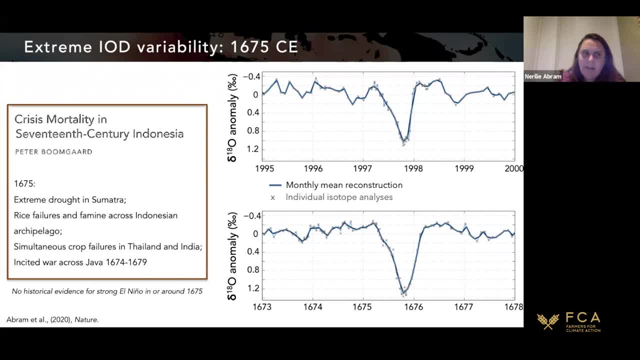 And so 1675 does stand out in those historical documents as being recorded as an extreme drought in Sumatra. There were rice failures and famine across India, failures and famine across Indonesia, and also simultaneous crop failures in Thailand and India, which meant that they couldn't import crops or food into Indonesia to help. 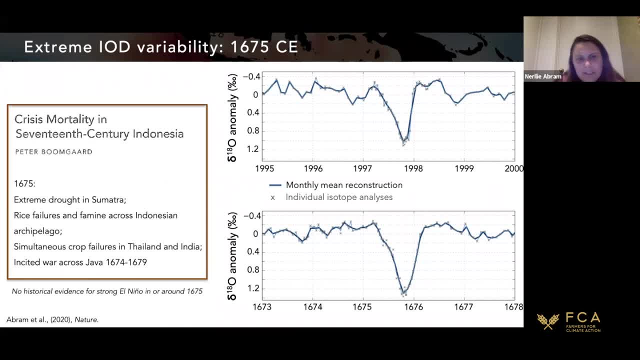 alleviate the famine there. Importantly, this is an event where a lot of these historical crisis events have been linked to El Nino events. in the past, This was an event that couldn't be linked to an El Nino event. there was no evidence of an El Nino event, and so here we see that. 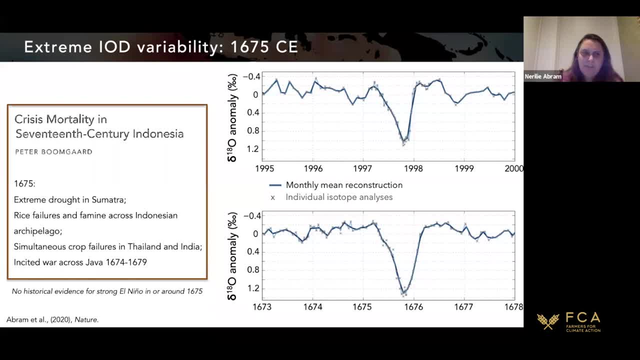 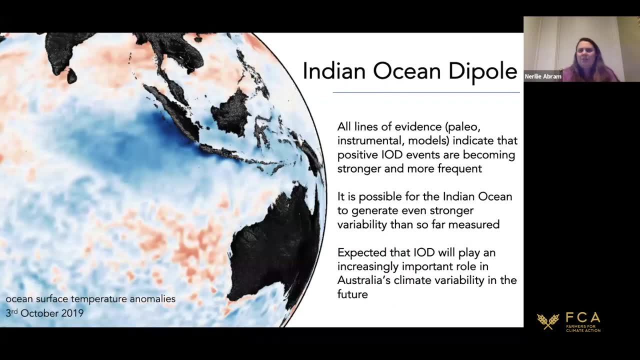 this was a case where the Indian Ocean was really sort of in overdrive and had some major impacts on the region. So a quick summary of where we're up to So with this new data. so all of our lines of evidence, so the paleo climate data, the instrumental data and the models, even with the uncertainties that 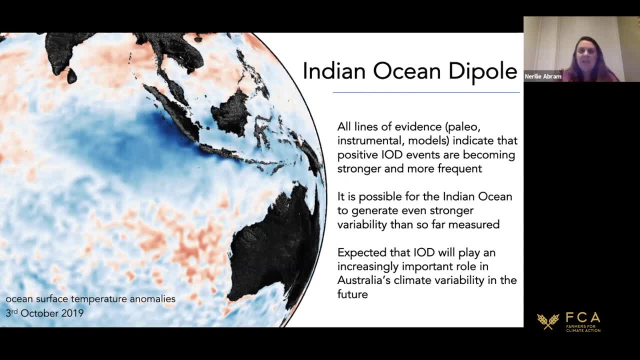 we have in those individual forms of evidence. they're all telling the same story. So they're all indicating that positive Indian Ocean dipole events are becoming stronger and they're happening more often. From our reconstruction we can also see that it's possible for the Indian Ocean to 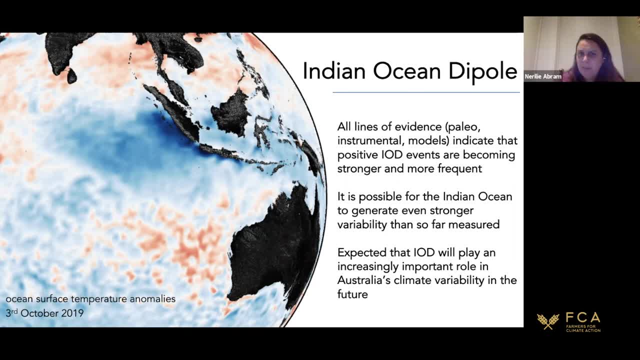 generate even stronger variability than what has so far been measured. So I think that's something that, scientifically, we need to keep that in mind when we're thinking about the impacts of these events and being aware that the instrumental record doesn't necessarily tell us about the full range of the impacts. that 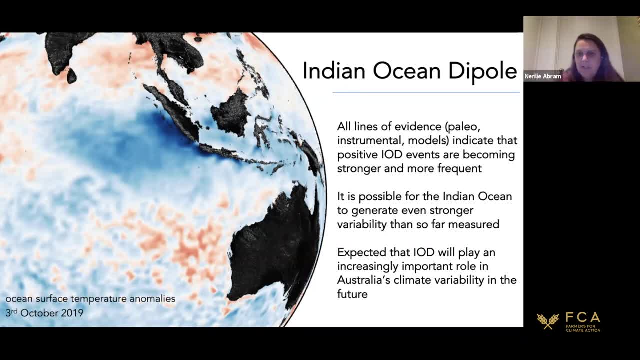 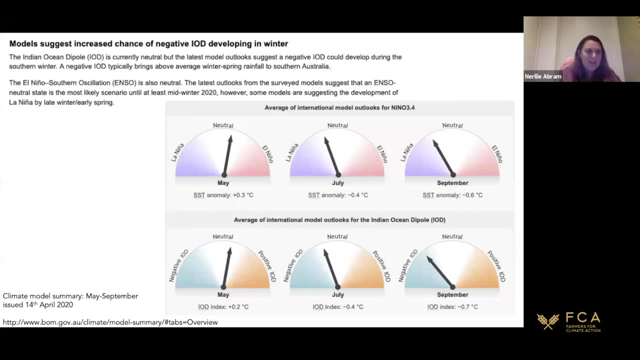 they may have, And we expect that the Indian Ocean dipole is going to play an increasingly important role in Australia's climate variability in the future, particularly if we continue on a high emission pathway. So what can we do? So I did mention that the Bureau of Meteorology does use the Indian Ocean dipole in 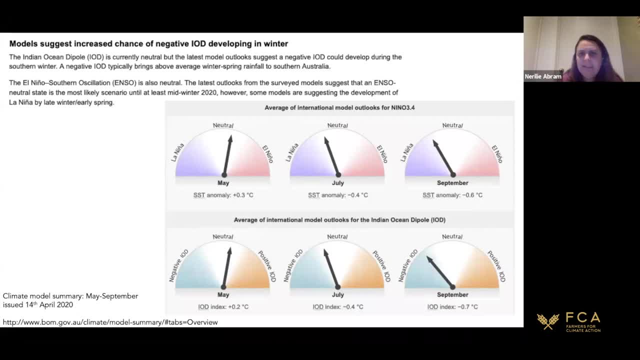 their climate outlooks. So this is the most recent climate model summary, issued just a couple of days ago, So this is a bit of good news in that at the moment, it looks like the Indian Ocean dipole is pushing towards a tendency to go to the negative state for this current winter and spring. There is some caution in that, and 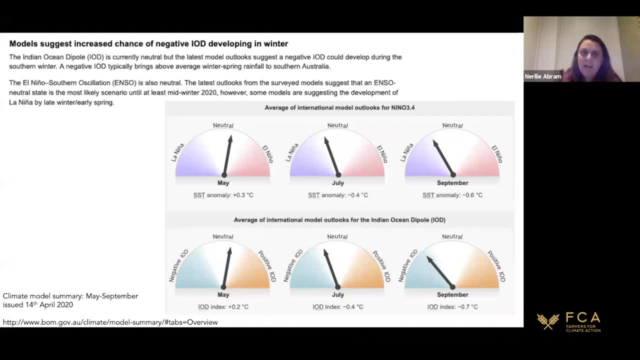 that typically this is a quite a hard time of year for making predictions of the Indian Ocean dipole and El Nino. Typically, once we get through into May, we start to have a clearer indication as to whether either of these climate modes is going to move into a positive or a negative state. 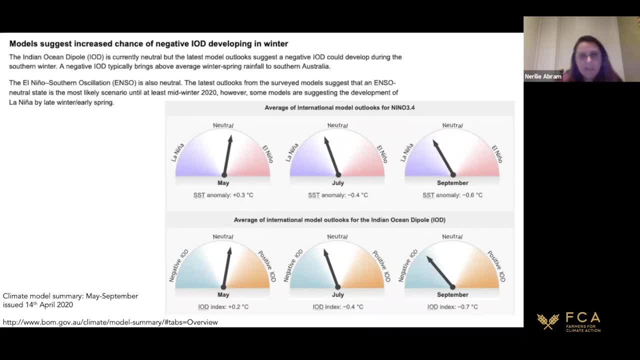 So it's still quite early to have a lot of confidence about this, but at least the needle's not pointing towards another positive Indian Ocean dipole event this year. So this is one thing that we can do is to look at, to take note of, the Indian Ocean dipole. 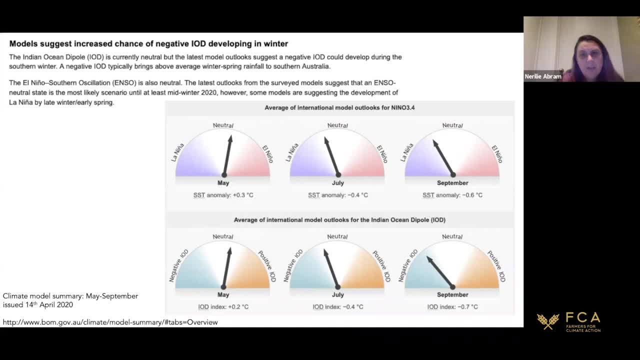 in those long range forecasts that are put out Scientifically. we've got work to do to improve those long range forecasts and to see if we can overcome some of those barriers that we have to sort of predicting sort of more than a few months out. 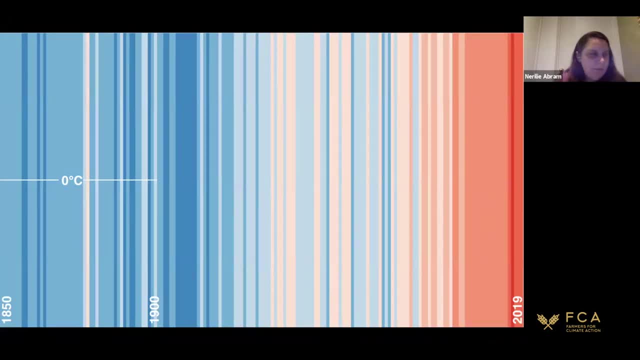 And then I just wanted to finish up with this. This is a type of image that you may or may not have seen before, So this is called a climate stripes diagram. So this is a visualization of global average temperature from 1850 through to the end of 2019.. And so 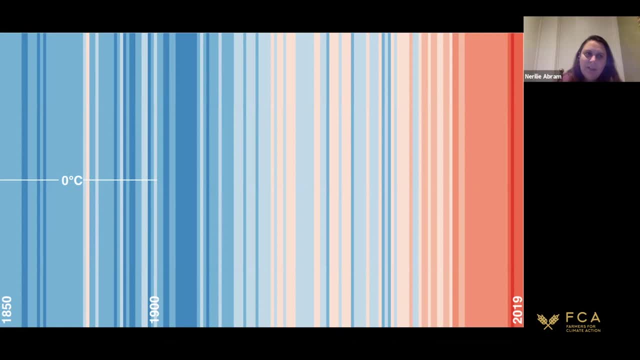 so in these climate stripes, every year is given a color based on the global temperature. We set the period from 1850 to 1900 as having an average temperature of 0 degrees. This is our what we call pre-industrial, And so this is the period of time where we hear about the Paris. 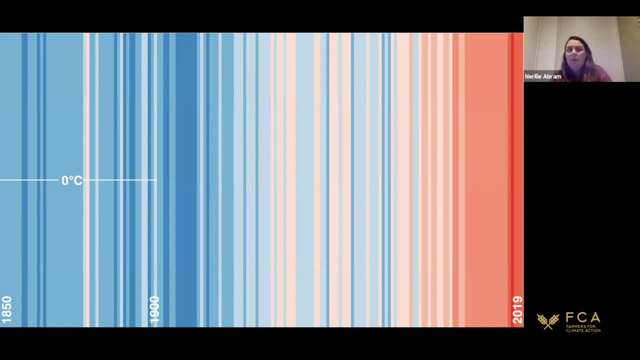 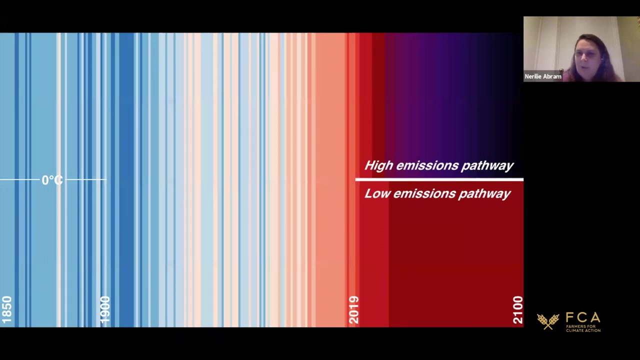 Agreement and trying to limit warming to no more than 2 degrees above pre-industrial. that 1850 to 1900 is that pre-industrial level, and so at 2019 we're sat with global warming at a little bit over one degree above that pre-industrial level. if we go and look at our climate models going through, 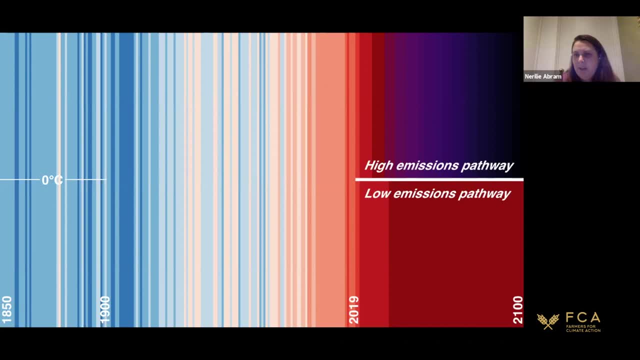 to the end of 2100. this is what that climate stripes diagram looks like if we choose a high emission pathway as opposed to a low emission pathway, and basically across pretty much every aspect of the climate system, a low emission pathway has lower climate risks associated with it compared to a higher emission pathway. the same is true for the indian ocean dipole. 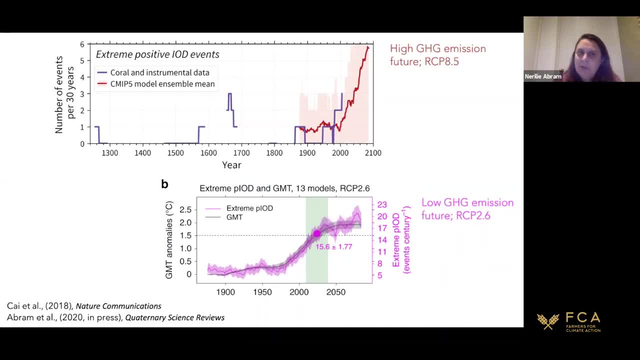 so in that top panel and this is just showing the frequency of extreme positive indian ocean dipole and this is just showing the frequency of extreme positive indian ocean dipole and events. so you can see that continuous increase if we continue on a high greenhouse gas emission. 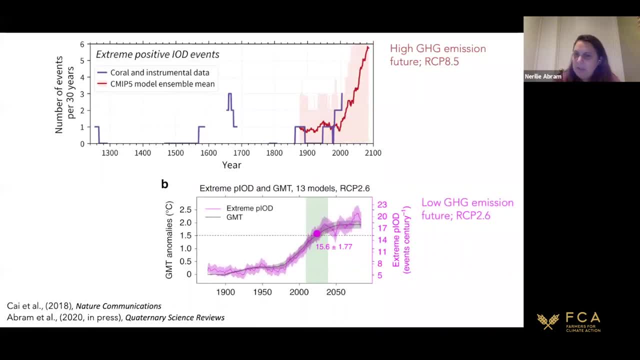 future. if, on the other hand, we choose that low greenhouse gas emission future, so rcp 2.6- we still see that increase in events becoming more frequent during the the 20th century and into the start of this century, but then we see a leveling off of that. so so this is a change where 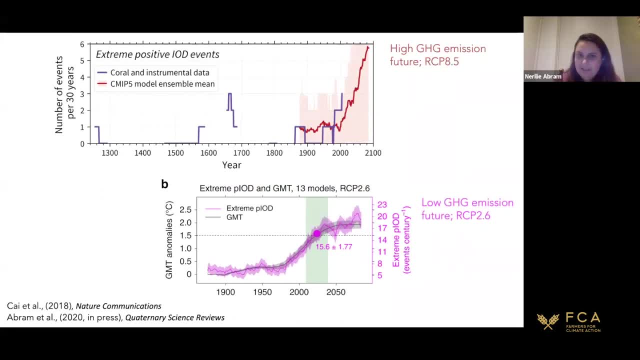 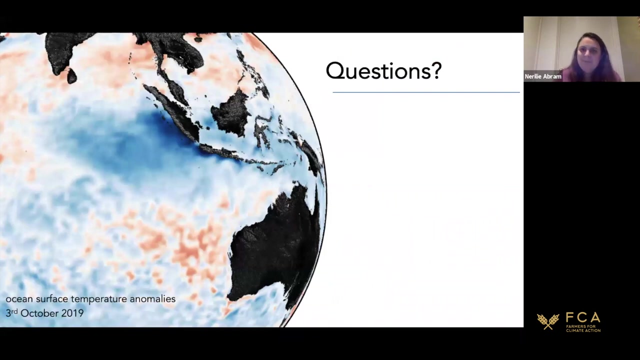 we do expect that positive indian ocean dipole events will continue to become more frequent. but we can limit how much that that change can, how much we let that that change continue on for right. so that was that was it in terms of the the presentation, happy to take questions. thanks so much for that narrowly. 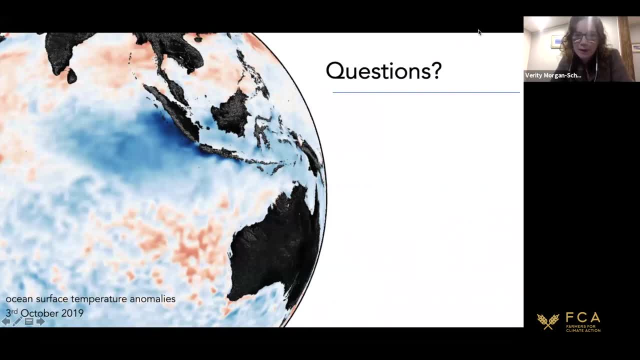 that was fascinating. so we've got a couple of questions that have come in from the audience. so we've got a question from peter over in the southwest of wa um, and peter's question has been: this: may or may not be related to the iod, but considering the huge impact of the climate, 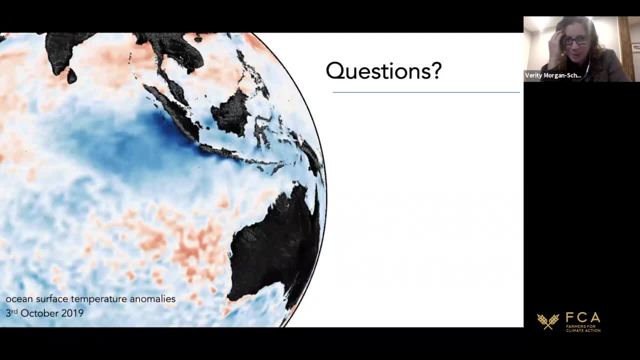 change induced wobble of the the arctic vortex has in the northern hemisphere. has the antarctic vortex had an impact on our weather and, specifically, has it or will it have an impact on the iod? yeah, that's a really fascinating question. um something, something that we're working on, um in. 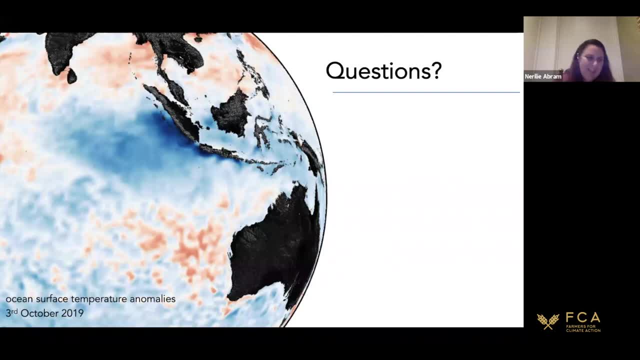 my in my research team to try and understand that from the last millennium perspective, um, so so what we're seeing, um with antarctica, um, is that the, the southern annular mode is becoming more positive, um and so so what that means is that, um, the, the mid latitudes have been warming up faster. 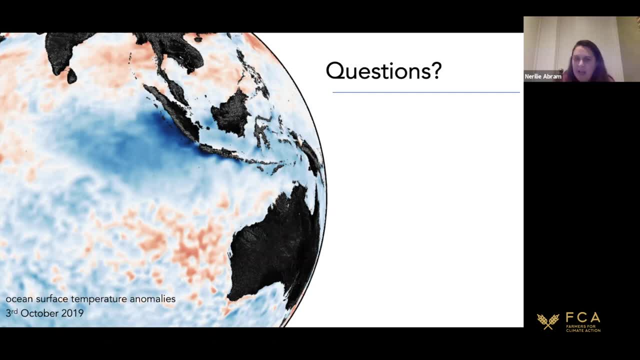 than antarctica. so we're increasing the temperature gradient, which is increasing, causing a positive southern annular mode, which means that the westerly winds shift further, further south um. so for for southwest wa, where there's been that really drastic decline um in winter rainfall, um that's an effect of the 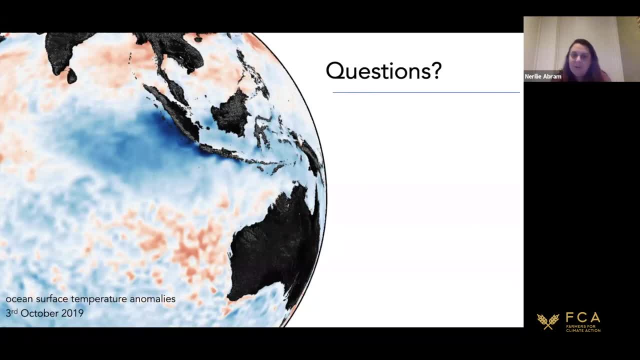 the southern annular mode and those westerly winds shifting further south, so so the rainfall that would normally come on those westerlies um, the westerlies are still carrying rainfall, it's just that it's not hitting australia because it's sitting too far south um so 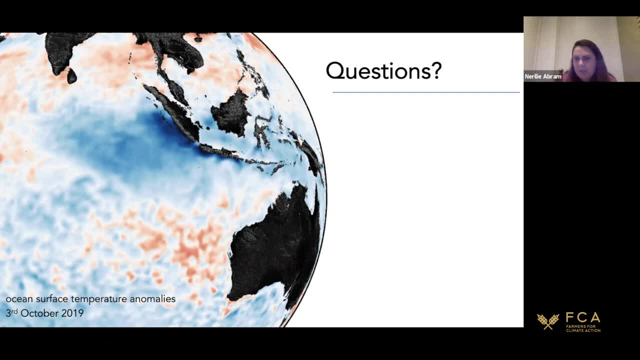 um. so into the future? um we do expect that in winter um the southern annular mode will continue to become more positive, you think um in the summer it's. it's a an interesting um trade-off between the recovery of the ozone hole um and those increasing greenhouse gases. so in the long 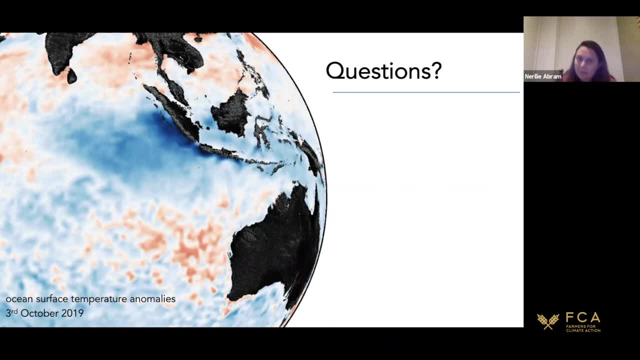 term. um, we do expect that the greenhouse gases are going to win um that that tug of war, and so we will see that positive um. you know we will see that positive um. you know we will see that positive trend continuing in the summer as well, um, but at the moment where we've got ozone recovery. 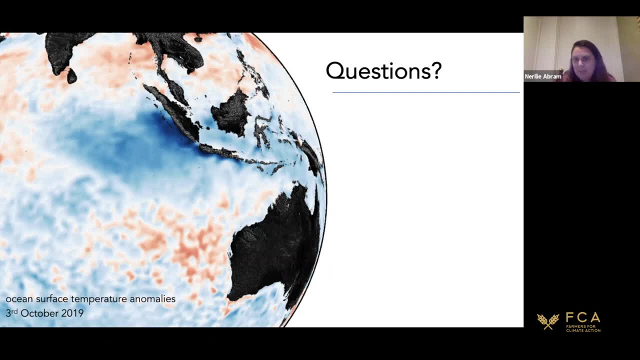 we're also seeing, um a slowdown in that positive trend and we would expect, expect that for for a few decades, um or so, um so. so it's a it's a difficult one um the the interactions are really interesting. there's definitely an interaction between the el nino and the southern annular mode. 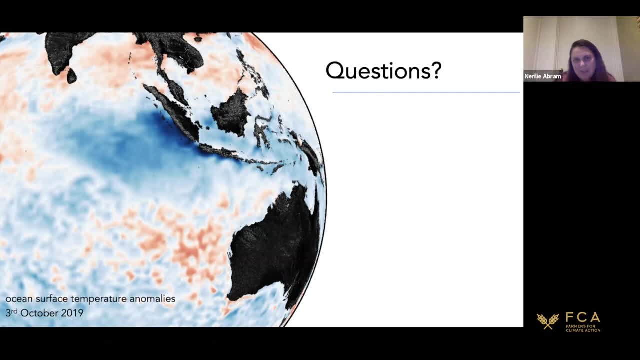 there's probably an interaction with the indian ocean, but we're still trying to understand it. thanks narrowly. and lucinda, who is not too far from holbrook in new south wales, has put a question around. what was the modeled temperature increase in the low emissions future? with the modeled 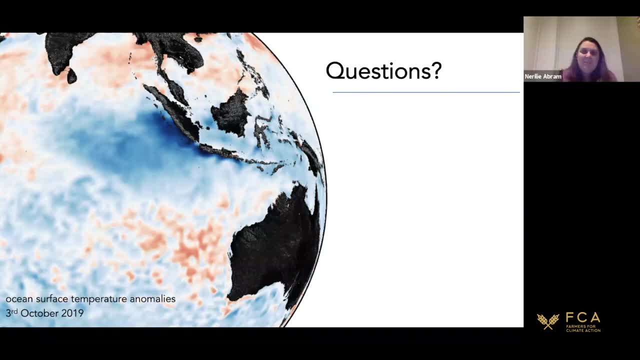 effects of the iod. um, yeah, so, so that, um the rcp 2.6, that low emission scenario, um, under that scenario, we end up with a around about a two-thirds chance of limiting global average warming to um two degrees. um, in that that high emission scenario, we're talking about more like four to 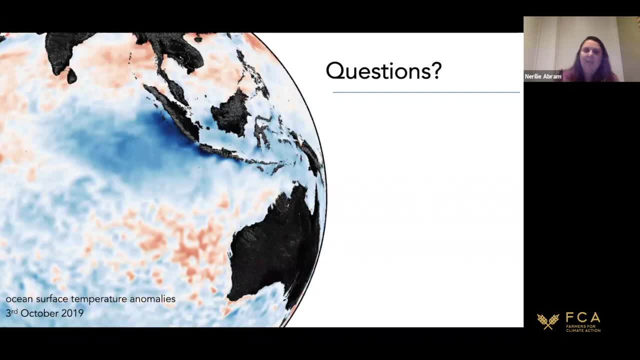 five degrees of warming by the the end of the century, and that being a a continuing trend, um beyond 2100 as well. um, yeah, so so sort of a quick answer on that in terms of what those global temperature levels compare to- beautiful. do we have any more questions that people haven't put in the chat boxes yet? 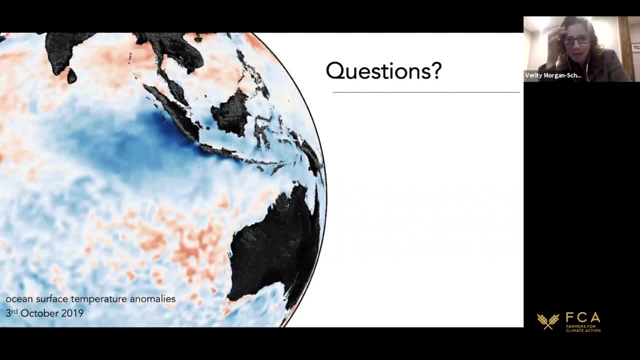 oh sorry, nick's got one. so nick's put a question around to the ocean heat waves that we are seeing cause the bleaching in the great barrier reef. do they have any potential to break down the positive iod or el nino events? um, i think that they're probably more of a side effect. um, of those, 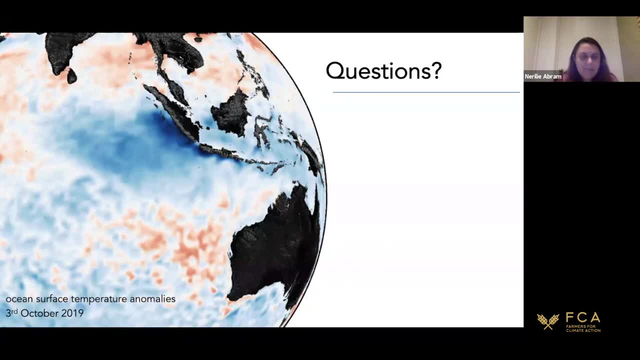 so yeah, so marine heat waves um are something that we're seeing happening everywhere in the ocean um when we, when we have the, the, those marine heat waves over a coral reef, that's when we get coral bleaching um. but we also see the impacts in places like offshore of tasmania, um the impact that that has. 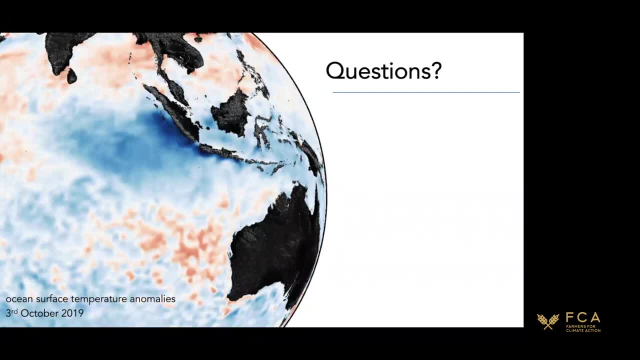 has on the kelp forest there, um and on the, the aquaculture industry, um, yeah, so, um. so certainly the, the um, the el nino and the indian ocean dipole will have an influence um in any given year. so, for example, when you have one of these positive indian ocean dipoles, you're going to have a lot of impact on the. 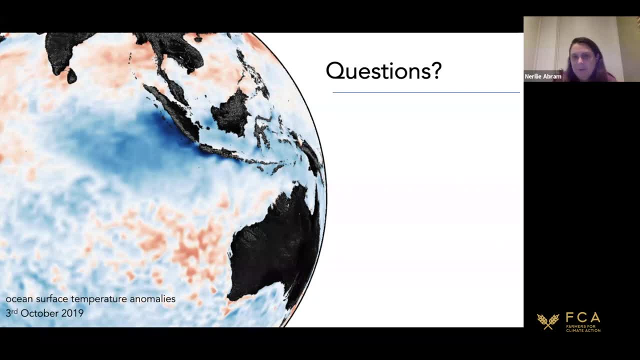 um the el nino and the indian ocean dipole events um like what's shown on the screen here, and you have those cool ocean temperatures off the coast of java and sumatra um those reefs in that year um are going to be sitting in relatively cool water and so they won't be um under that same. 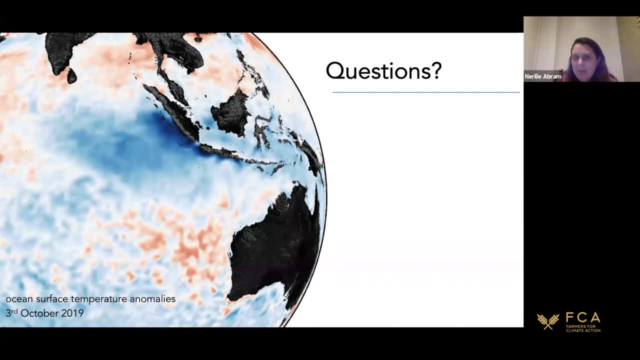 risk of bleaching um. but if you turn that around and move into a negative indian ocean dipole event, that water becomes warmer and so you increase the risk of bleaching um. so so it's more, it's more the those um climate modes, um and the el nino and the indian ocean dipole events are going to be. 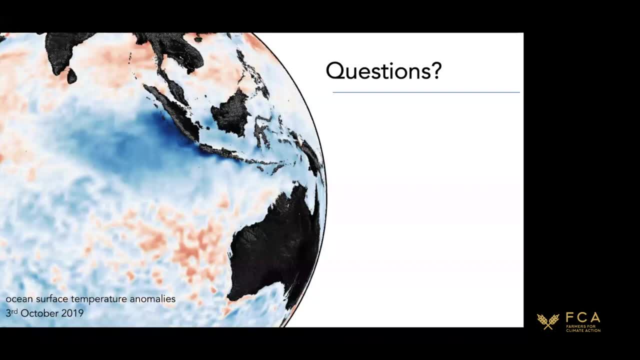 affecting your chances of having a marine heat wave and the bleaching in that reef environment, rather than the other way around. thanks, narrowly and nearly. we've got a couple more flowing through, which is great. charlie has put one which is very close to my heart at the moment. my home farm was 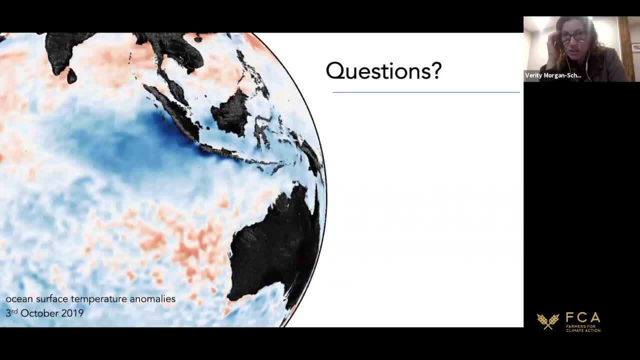 decimated and the childhood home destroyed about six weeks ago through a mini cyclone in wa. and so charlie's question has actually been: do you have any data on the relationship or a relationship between the iod and cyclone in the indian ocean? um, not directly. um, there there is a link with with el nino, but generally, 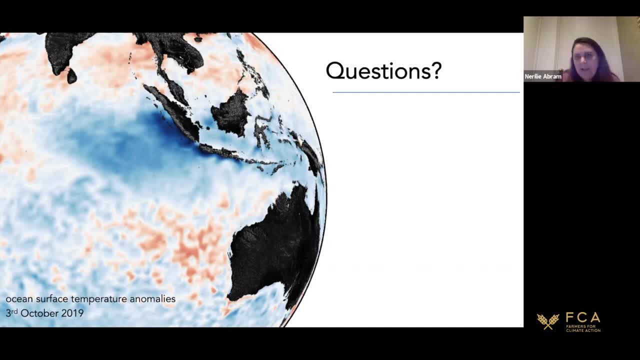 what we see um is that when we have um warmer water, then we're more likely to have have cyclones, and so what we saw in the indian ocean in this last year is that once the once the um. well, so when we had the positive indian ocean dipole event happening um the eastern indian ocean, 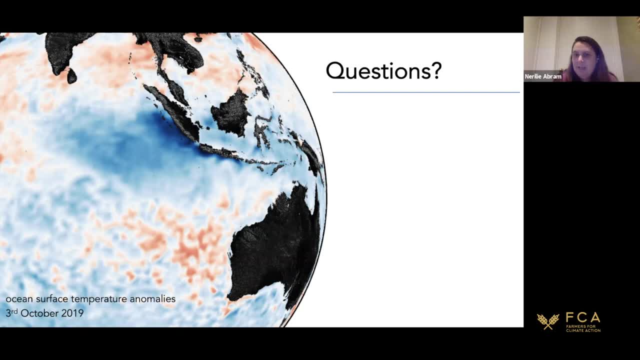 was unusually cool, but the western indian ocean was unusually warm, and so there were places in eastern africa, um, and and up into the middle east, that experienced cyclones there, where they wouldn't normally have experienced cyclones, and that was because you had those warm ocean temperatures, um. and then what we saw once the indian ocean dipole, um, broke down- um, in december. 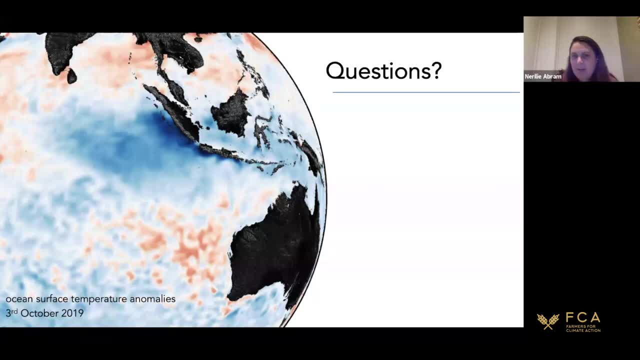 that allowed the eastern indian ocean to start warming up and that's where we started to see cyclones then developing um off the northwest of australia and that's um one of the one of the factors that contributed to that rain that came through in february, um and finally sort of put. 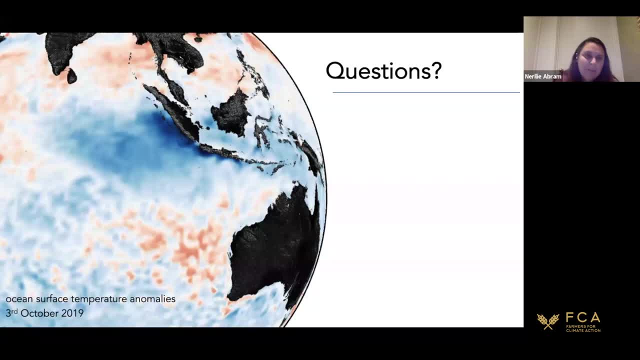 out the fires in eastern australia as well. um, so yes, there is a link um between um these events, um, it's, but it's better studied so far for el nino, um and showing sort of the link between el nino and la nina years in terms of where you're getting cyclones and how. 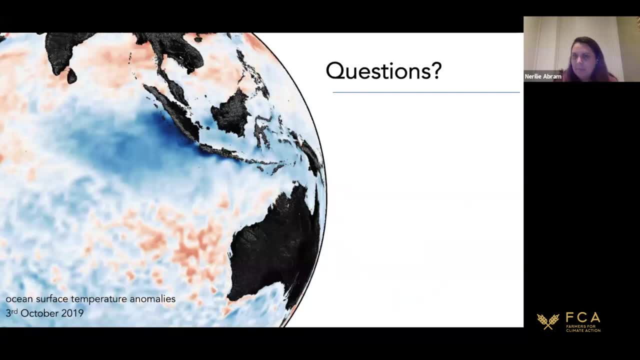 um, how frequent you expect cyclones to be that year? fantastic, nearly. i'm just very conscious of time, so we might take three more questions, if that's okay, so we don't keep you too late. um, so we've got a question about the, the physical mechanism. 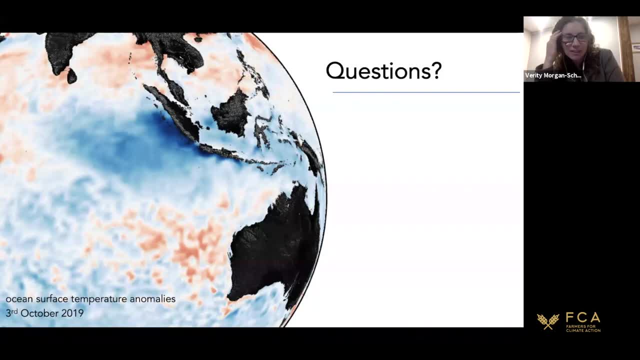 by which a positive iod affects southwest australian temperature, um, yeah, so so again. so what we have, um when we have a positive indian ocean dipole there's, there's two, two factors that go on there in terms of the, the temperature, um particularly into into southwest australia. 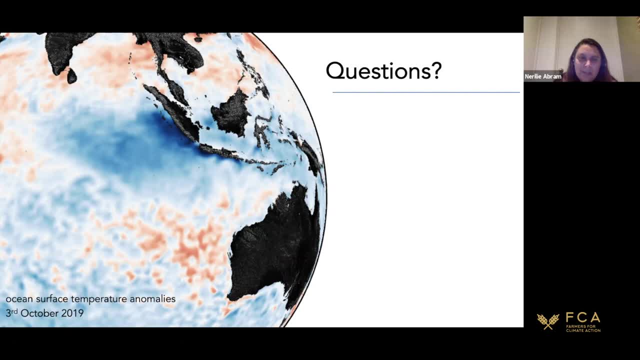 um. so what you can see- um it's actually quite nicely shown on this image- is we. when we talk about the indian ocean dipole, we talk about positive events, having cool ocean temperatures in the eastern indian ocean, eastern tropical indian ocean and warm ocean temperatures in the. 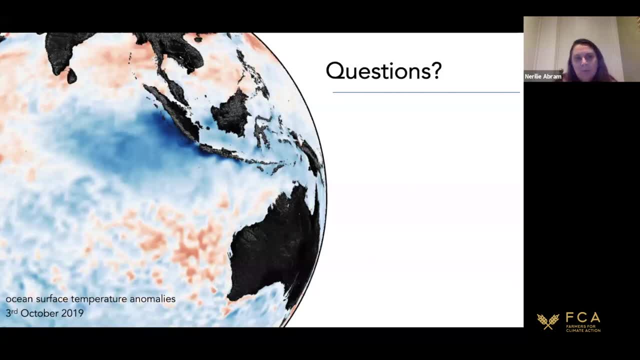 west. so we talk about that east west gradient um. but those warm temperatures in the west um tend to sort of have a horseshoe pattern around the cool anomaly, and so you can see those that warm water that sits um off the the southern coast of western australia. 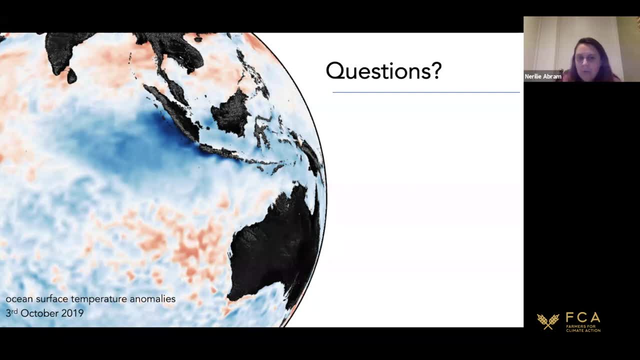 so you've got, typically during these events, um quite warm water off the southern parts of australia, so that will make the climate um onshore a lot warmer um. the other thing that's happening is that we've got um the air that's drawn down from the northwest across australia um being very 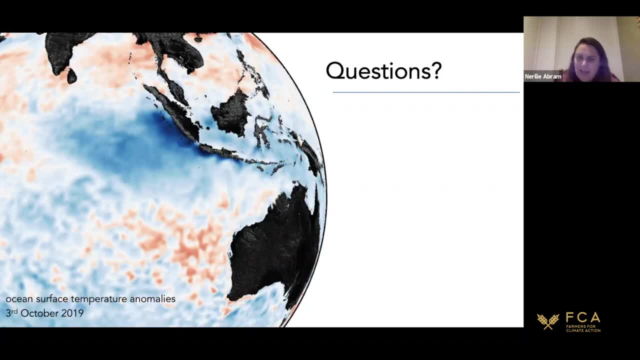 dry um, and so when we have that, that dry air, we're not able to take up as much, we're not not able to to transfer as much of the the incoming radiation that we get from the sun um, we can't change, take up that energy through evaporation, because we've got very dry air and so that allows. 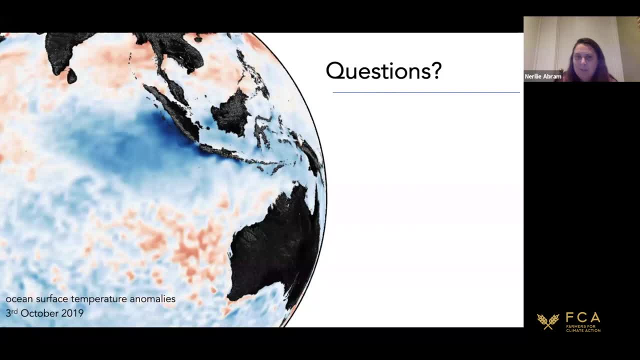 that air to to heat up more. um, so it takes that energy in and puts it into changing the temperature of the air rather than evaporating water instead fascinating, um, so nearly just a couple more we've got. so, um, pete's raised the question of the the 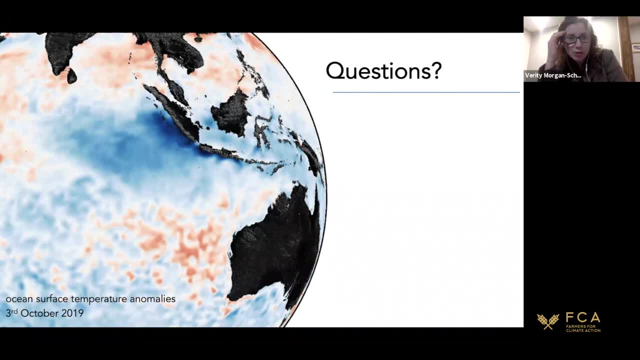 depth. does the depth or the volume of the indian ocean alter its heating potential? i understand the indian ocean's relatively shallow as oceans go, so does it alter its heating potential under global warming and will this affect um current circulation and therefore the iod strength and impact? is that able to be modeled at this point? um, it can be. it can be modeled um the indian ocean. 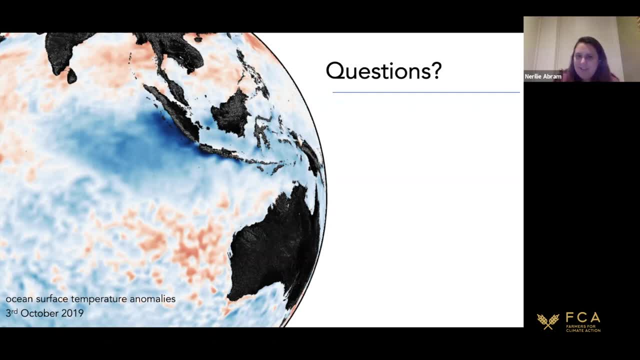 is actually one of the the ocean basin that's warming sort of faster than any other, any of the other basins, um, but generally. um, yeah, when we're talking about sort of ocean heating, we're talking about sort of the upper, um, the upper sort of hundred meters or so of the ocean, and then that gradually sort of gets. 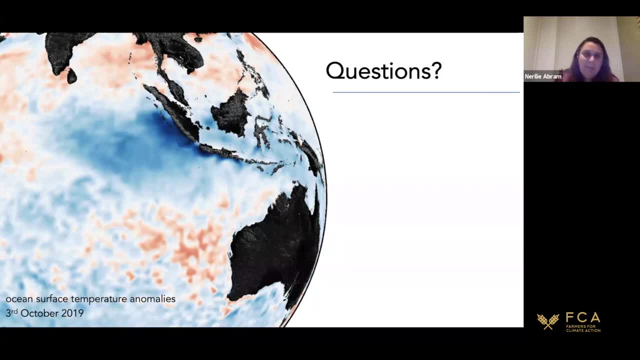 circulated into deeper levels of the ocean? um. the ocean is enormous, and so it's able to take up a huge amount of heat? um, and it does take up a huge amount of heat? um, but what we're seeing in the in the surface ocean, is that the, so the indian ocean um is warming very fast, but it's warming faster in the western. 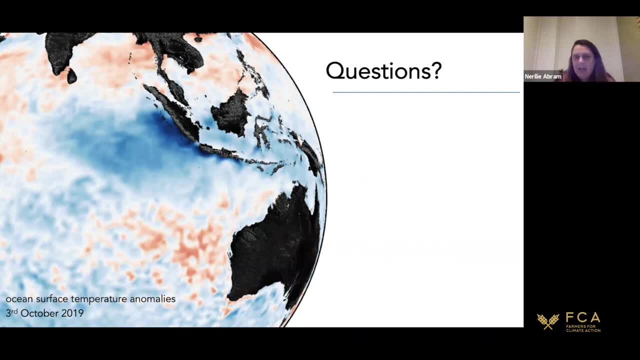 um side of the indian ocean to the eastern side, um. so so we're seeing sort of a sort of the average condition of the indian ocean moving towards this sort of more positive indian ocean dipole state, and that's one of the factors that means that we're seeing these um. 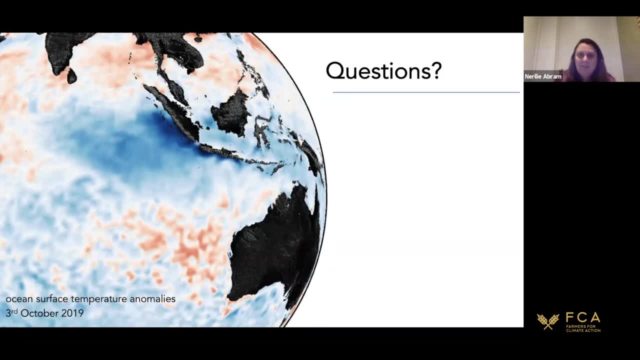 these events happening more often because of the way that global warming isn't warming, or ய um izes um. so i think that's where it's joining the um um um lot of positive events, and we saw that particularly strong 1675 event. So, yes, this was part of. 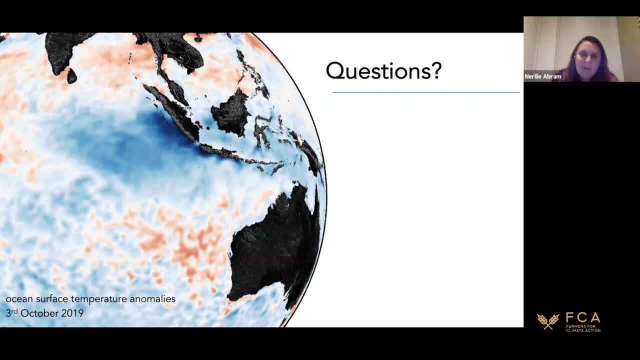 the natural variability that we can expect. There was a period of time that you'll sometimes hear referred to as the Little Ice Age. So generally, climate was cooler at this time, But what happened in terms of the average climate was that the oceans around Indonesia 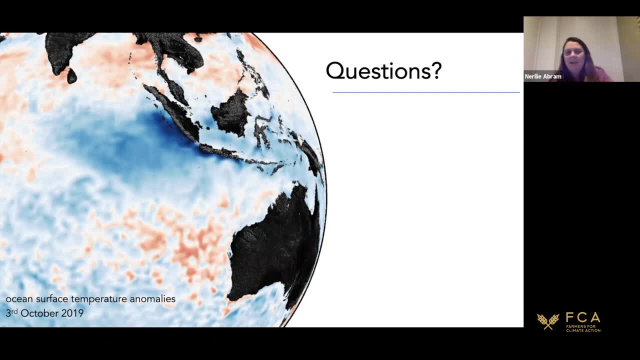 cooled more than other places. So again, like I was talking about, at the moment we're pushing the Indian Ocean towards the more positive Indian Ocean, like mean state, because we're warming the western Indian Ocean faster than the east In that period of time. 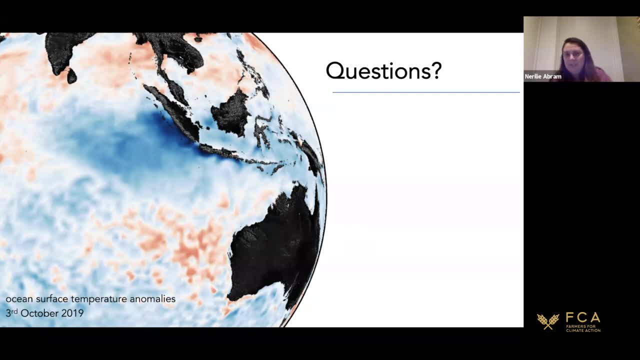 we cooled the eastern Indian Ocean more than the west and so the effect was the same in terms of changing that ocean temperature gradient, More like a positive Indian Ocean state, and made it easier to have those individual events. so different, different process, a different mechanism with the same effect on making those events more common. thank you, marilee, and final. 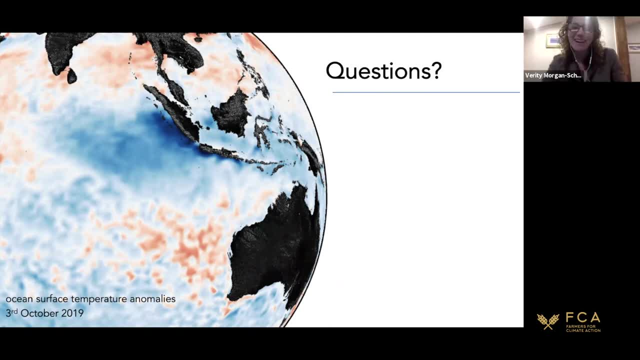 question before we we wrap up and let you go for the night. um, this one comes from carl young, who's down in the mildura region, and carl's question is sort of looking to the future a bit more rather than the past, and he's raised the point of if geoengineering occurs, ie the sulfur dioxide. 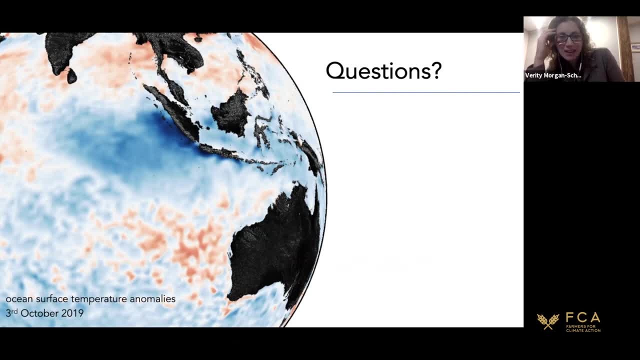 proposals. will the deposits be spread around or would it be localized? and if localized, would it be likely deposited in the southern hemisphere? so a little bit different to our previous conversation, but would love your thoughts on it. um, yeah, so so the the idea of um putting some sulfur, um. 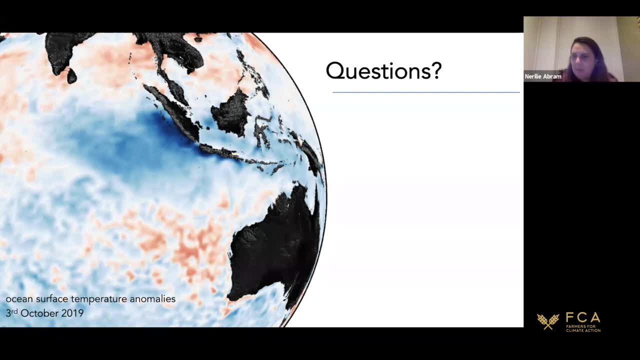 into the the atmosphere. so it's kind of simulating what we would have if we have a very large volcanic eruption. so to get that climate effect you really need to push, um, do that, inject that very high in the atmosphere, so like when you have a very big volcanic eruption, um. 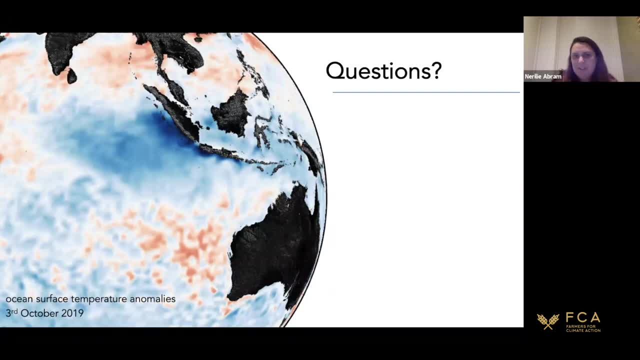 once you have sulfur up into that level of the atmosphere, it does sort of spread um all around the globe, and so we would expect the fallout to be seen all around the globe, and that's actually one of the interesting ways um that um, as climate scientists, that we reconstruct. 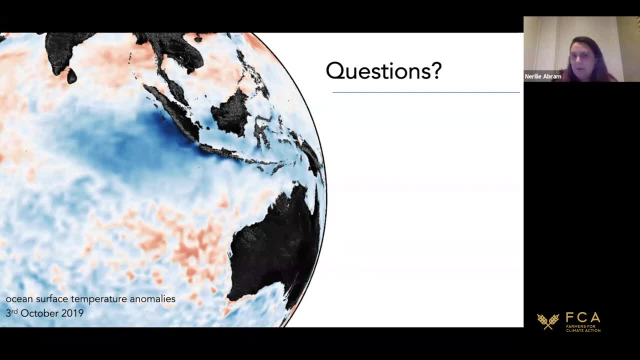 um, when these big eruptions have gone off in the past- and quite often these are tropical eruptions- um, but, what we're trying to do, is we're trying to do, is we're trying to do, is we're going to do, is we're trying to do, is we're trying to do, is we're going to. 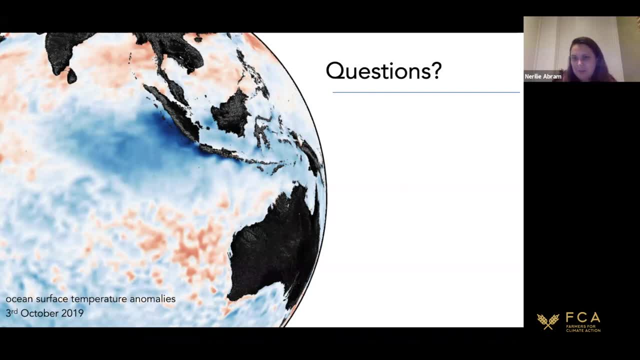 see what happens when we're into an eruption, um, so we'll be able to see several different forms of sulfur and we'll be able to see its incidence over time. so again it's it's a lot of time затanglement. so many of us are trying to figure out what we see, um and and so what we see. 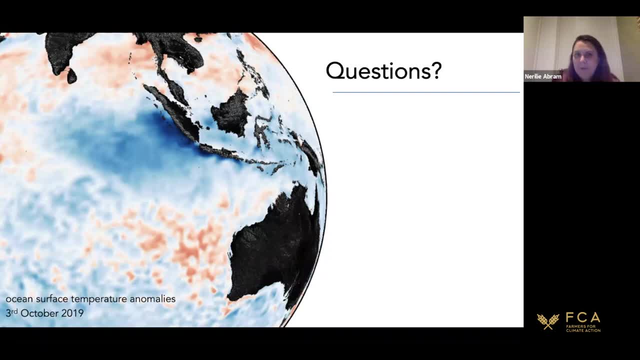 is. we see those sulfur deposits um in greenland ice cores and antarctic ice cores, and we see them in both of those ice cores at the same period of time, indicating that sulfur has gone all the way around the world, so injected at the tropics but then falling out all across the world. 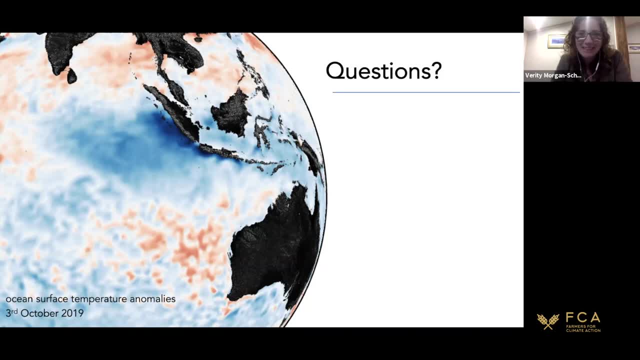 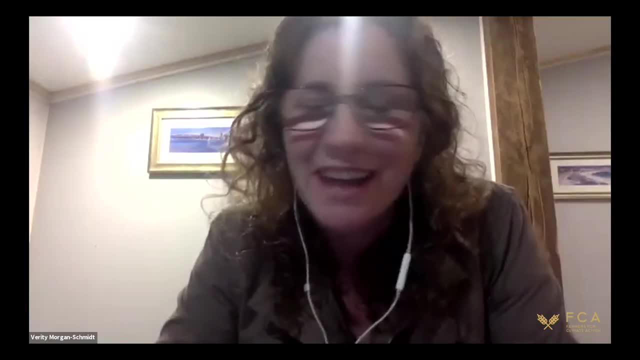 hand back to lucinda to do a thank you. i'll just acknowledge the other members of our team that are on tonight. so we've got wendy cole and fca's ceo, who's joined us, which is wonderful, and we've also got james atkinson, and then we've had farmers from all around australia, so it's been fantastic. 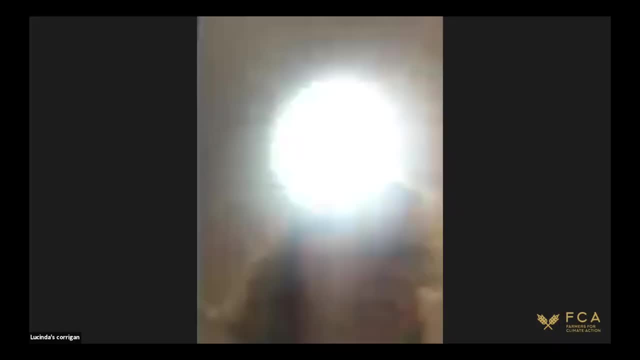 and nearly. thank you for um for agreeing to do this. lucinda, over to you for the formal thanks. oh look, nearly. thank you so much for sharing um. well, firstly, uh, your work over a thousand years, which is stunning really, just getting the understanding of um, some of the work you're. 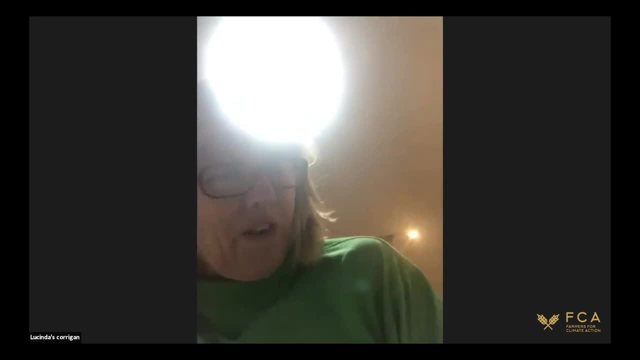 doing in the mentui islands and um those coral cores and thinking about what might happen with these models for the next um 80 years, which always sort of sets me back in my tracks when i think about my family and and um the sixth generation- my granddaughter's now born, and thinking about 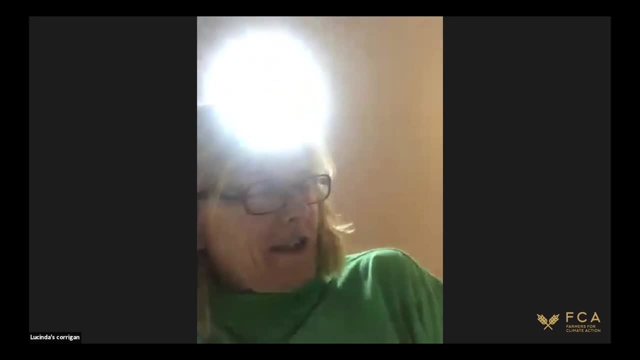 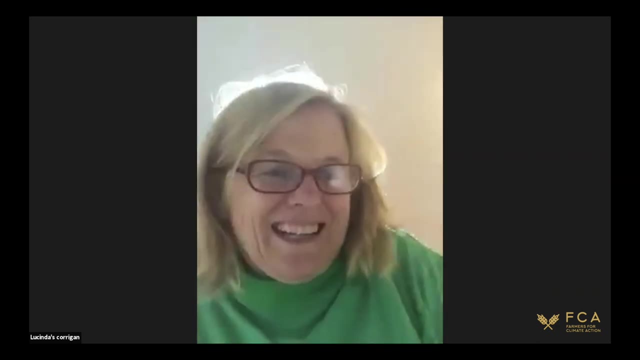 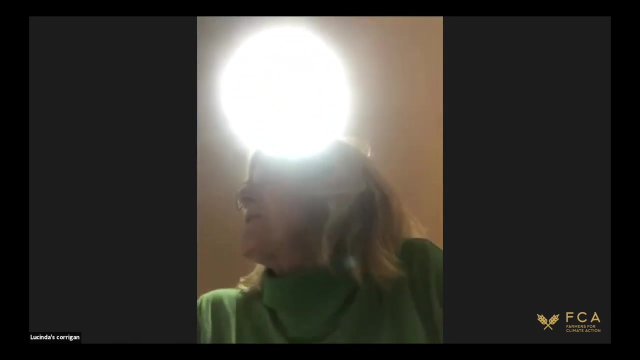 them still being alive in 2100. so it spurs us on to do what we do and to find a way to to well convince, i guess, the rest of society that we need to um to embark upon a low emissions future. but so interesting. thanks so much for sharing and i'm sure everybody tonight is delighted to have. 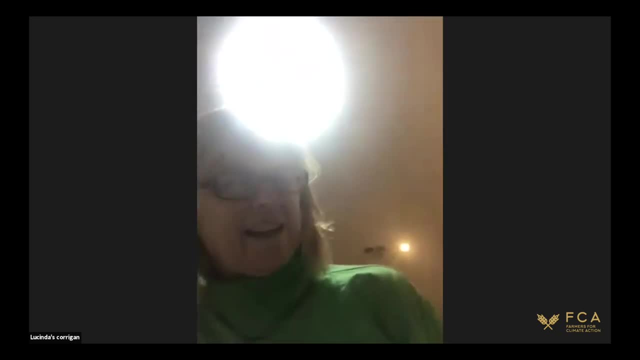 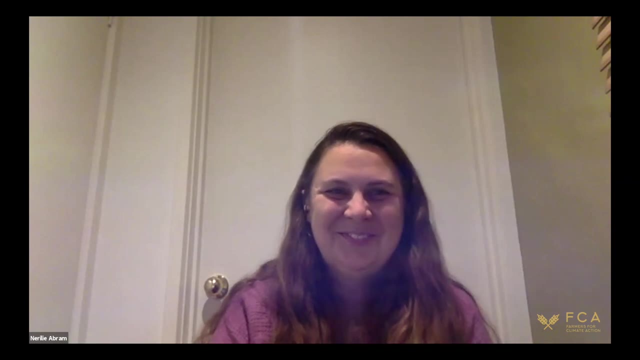 a chance to talk with you and listen to your experience. and congratulations on the paper for nature. that's just fabulous. thank you very much. lovely. thank you, lucinda, just before we go. um, we're just about to put a poll up on your screen. we just. this is the first in our series. 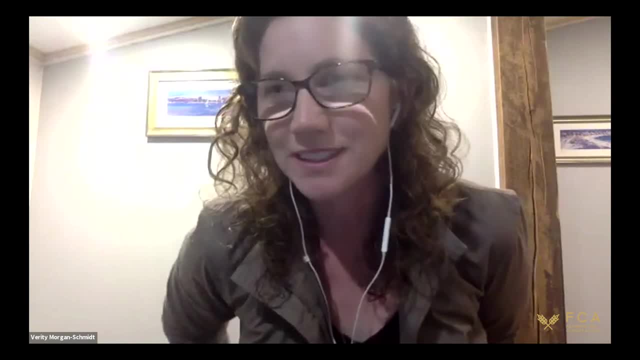 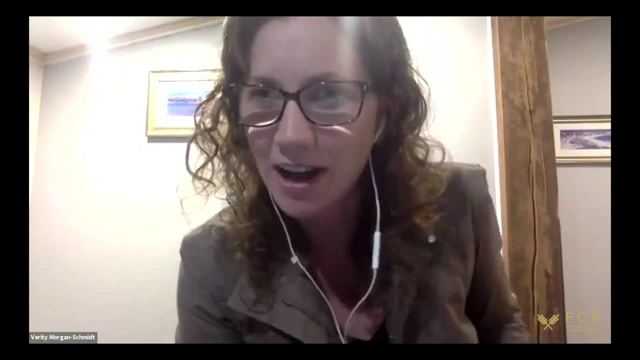 of webinars everyone. we'd really love your insights on how we can do this better, how we can best meet the um, the needs of our audience, particularly in relation to time, because it's a very live issue within our team. so if you could just quickly answer those two questions, i'd really.